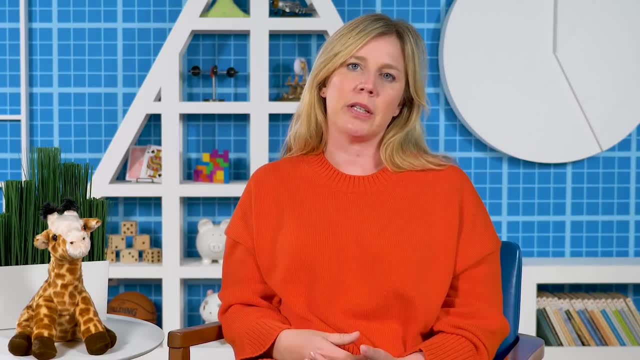 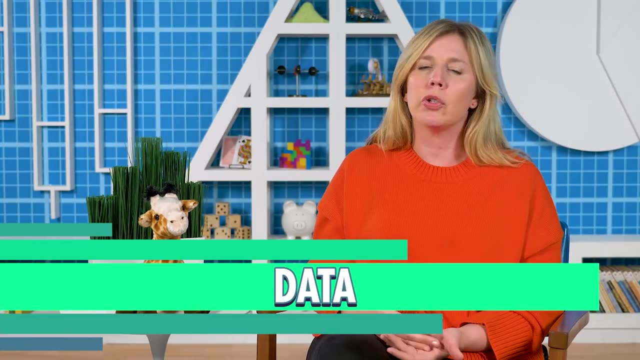 But I need to test my hypothesis. I can't just have an idea and claim it's correct without any evidence. One thing we need for sure is data, So we could randomly sample two groups of 25 people and make half of them listen to Mozart and half do their homework in silence. We collect. 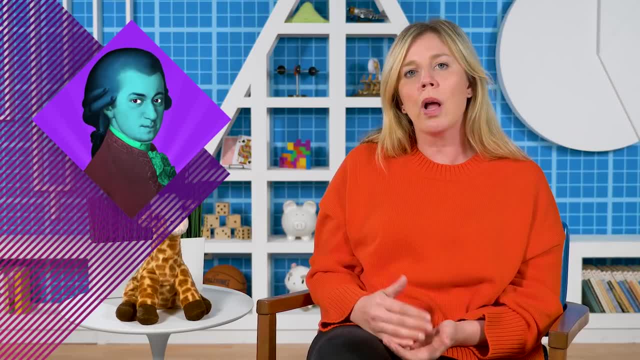 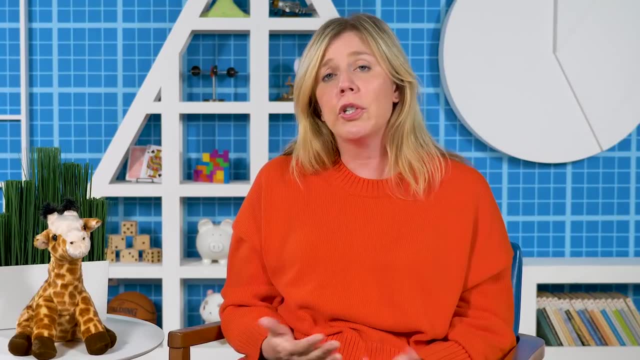 their calculus grades and see that those who listened to Mozart scored on average 3 points higher than those who didn't. So Mozart's good Problem solved: Break out sonatas right. Unfortunately no, We've seen that sample parameters like the mean and average score. 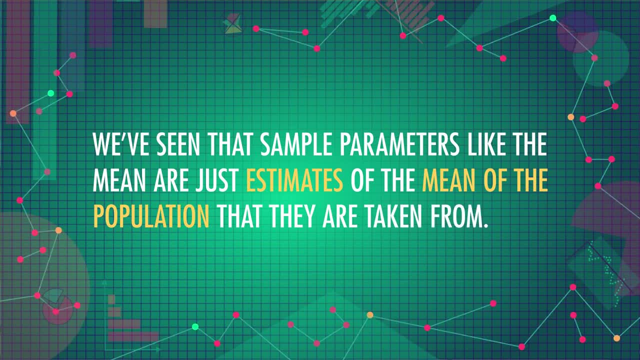 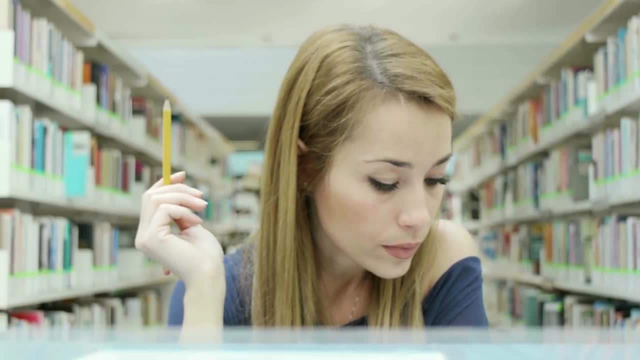 mean are just estimates of the mean of the population that they're taken from. The sample mean score of the Mozart group is higher, But we don't have sufficient evidence that the population mean of Mozart listeners is higher than those who did their work in silence. 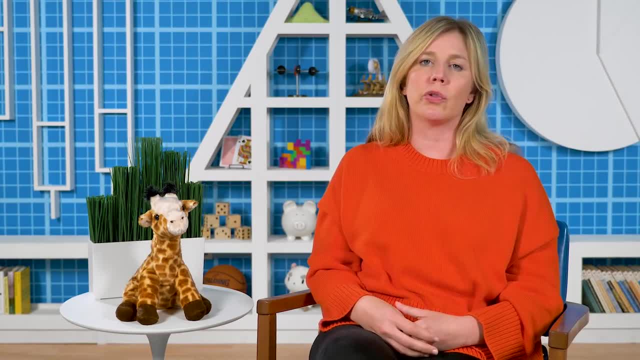 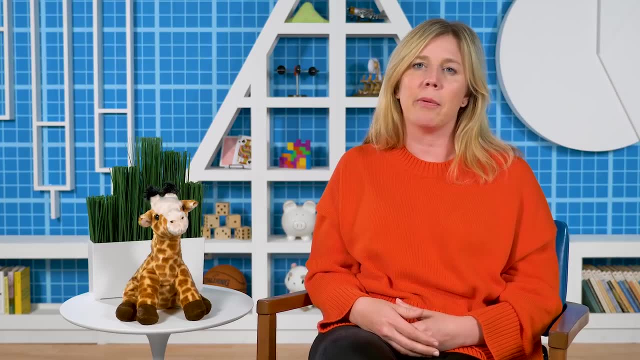 We may have gotten an especially high sample mean that isn't close to the true population mean. So we need a way to test our hypothesis while taking into account the random variation of sample means. In theory, one way you could test a hypothesis or model is by how well 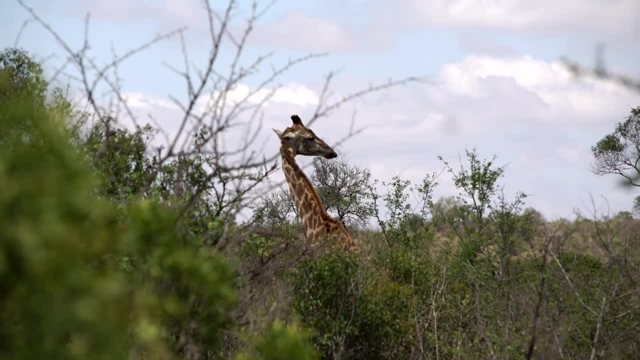 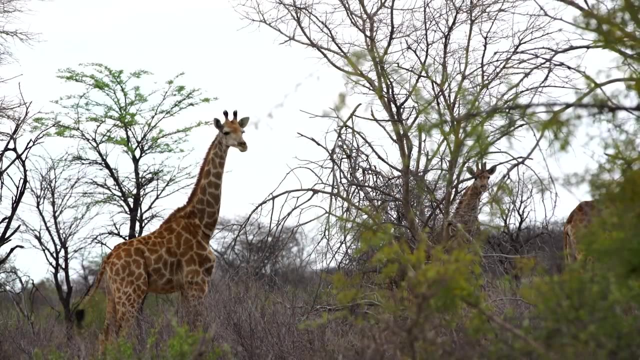 it predicts the data you got. For example, you and your best friend really love giraffes and you spend a lot of time watching them at the zoo and drawing sketches of them, So you both have a hypothesis about the average number of spots a baby giraffe has. but they're. 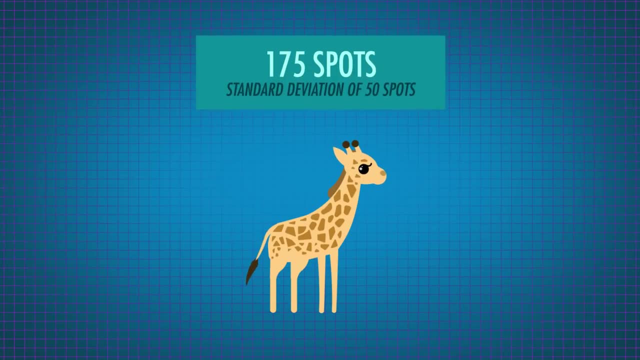 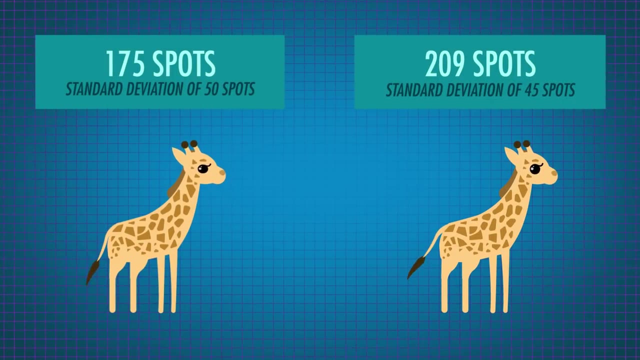 slightly different. You think that baby giraffes have an average of 175 spots, with a standard deviation of 50 spots, And your best friend thinks that baby giraffes have an average of 209 spots, with a standard deviation of 45 spots. With the permission of your local, 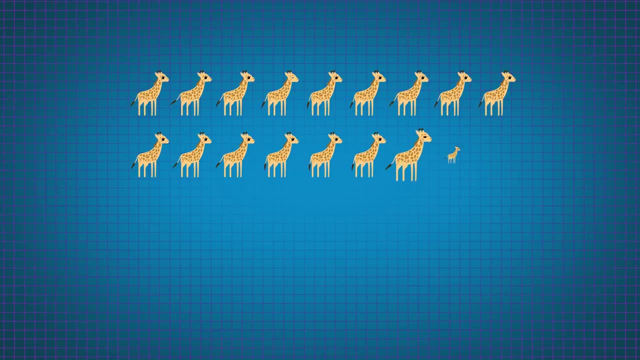 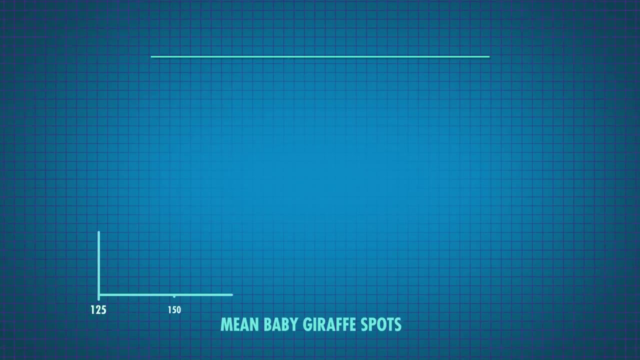 zoo. of course, You begin to collect a random sample of baby giraffes and count how many spots they had. Your sample of 25 baby giraffes had a mean of 200 spots. Now that you have the data, you can use it to evaluate which one of you is more likely. 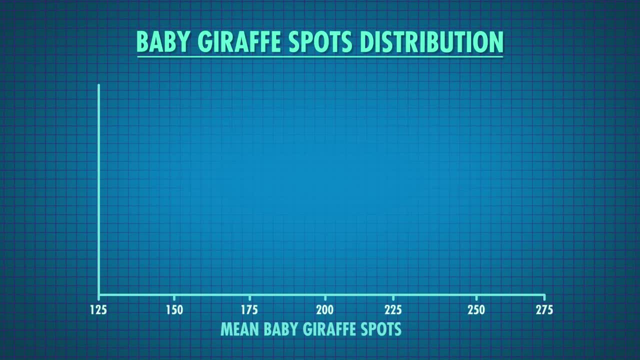 to be right. Both you and your friend have a model or idea about what the population distribution of baby giraffe spots is. If you're right, then the sampling distribution of all the possible sample means we could get looks like this And the distribution: 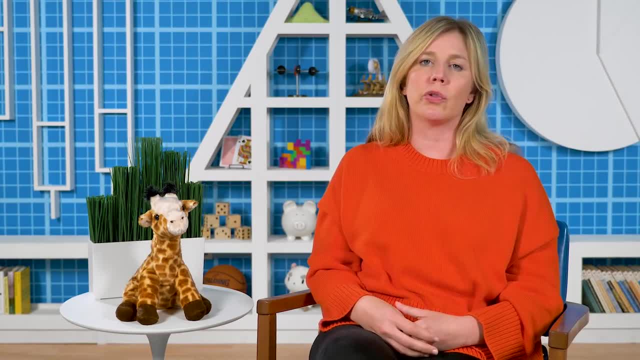 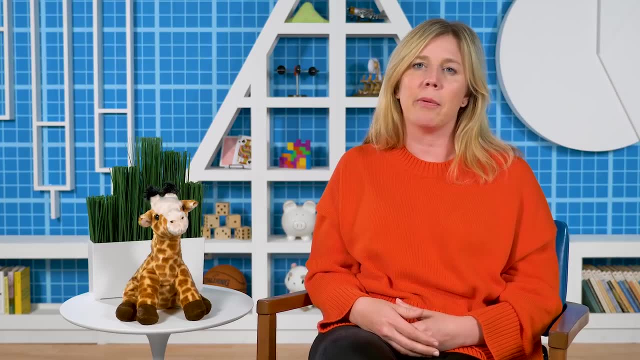 We may have gotten an especially high sample mean that isn't close to the true population mean. So we need a way to test our hypothesis while taking into account the random variation of sample means. In theory, one way you could test a hypothesis or model is by how well 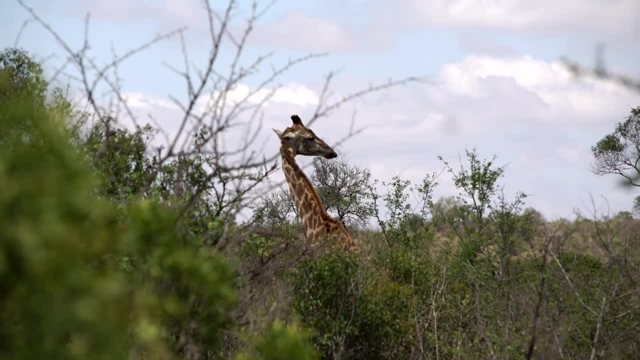 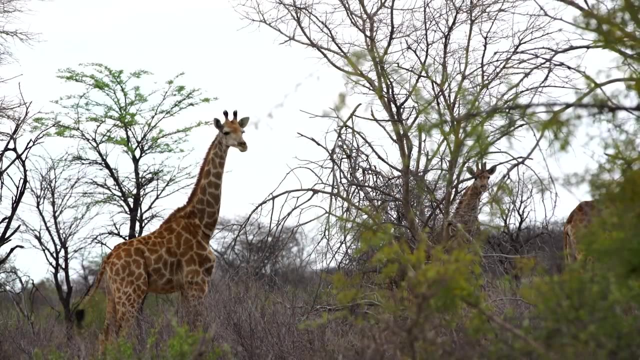 it predicts the data you got. For example, you and your best friend really love giraffes and you spend a lot of time watching them at the zoo and drawing sketches of them, So you both have a hypothesis about the average number of spots a baby giraffe has. but they're. 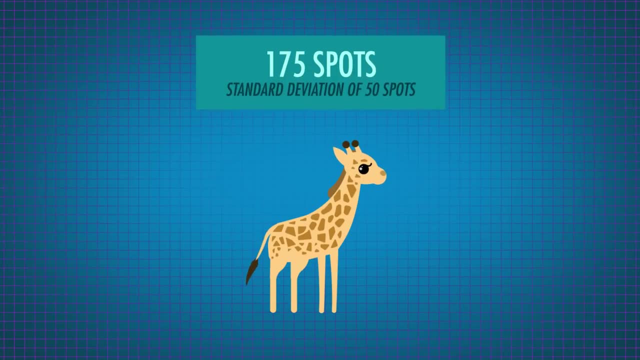 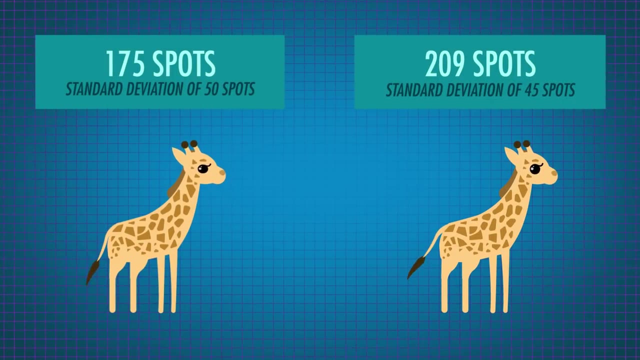 slightly different. You think that baby giraffes have an average of 175 spots, with a standard deviation of 50 spots, And your best friend thinks that baby giraffes have an average of 209 spots, with a standard deviation of 45 spots. With the permission of your local, 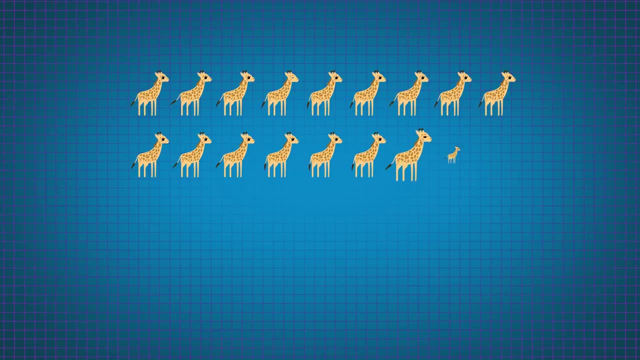 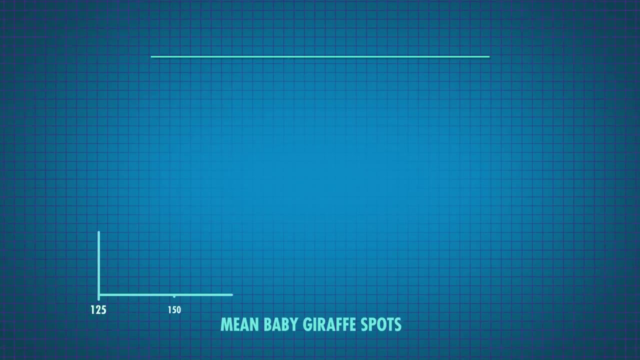 zoo. of course, You begin to collect a random sample of baby giraffes and count how many spots they had. Your sample of 25 baby giraffes had a mean of 200 spots. Now that you have the data, you can use it to evaluate which one of you is more likely. 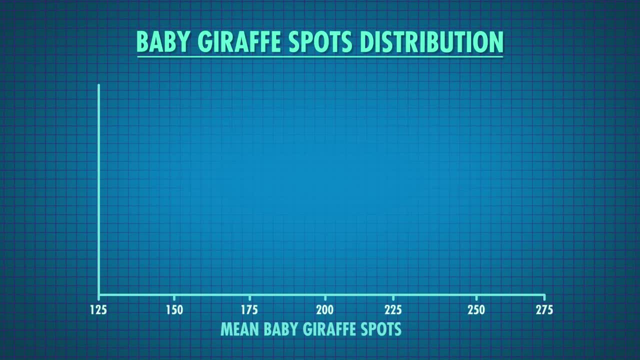 to be right. Both you and your friend have a model or idea about what the population distribution of baby giraffe spots is. If you're right, then the sampling distribution of all the possible sample means we could get looks like this And the distribution: 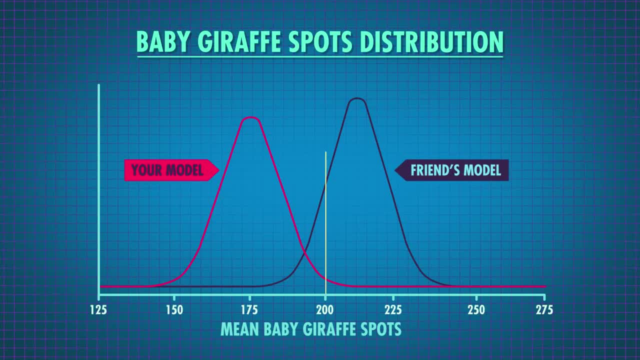 of sample means for your friend's model looks like this: Let's look at where our sample mean of 200 lies on both of these distributions. You can see that we're more likely to get a mean of 200 spots under your friend's hypothesis. 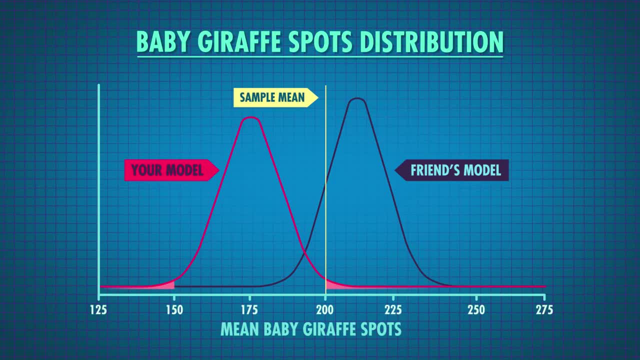 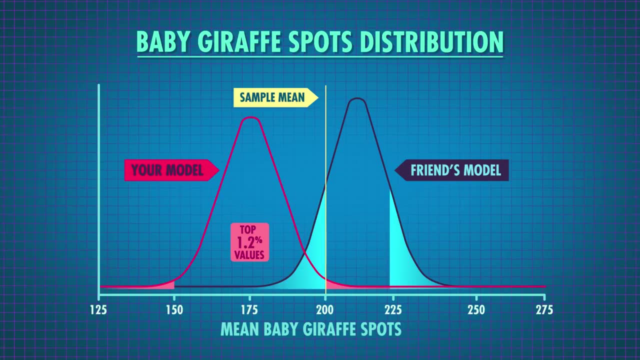 than yours. If your model were correct, a mean of 200 spots is pretty rare. It's in the top 1.2%, most extreme values we'd expect to see, Whereas in your friend's model a mean of 200 spots is only in the top 32%, which means it's pretty common that we'd 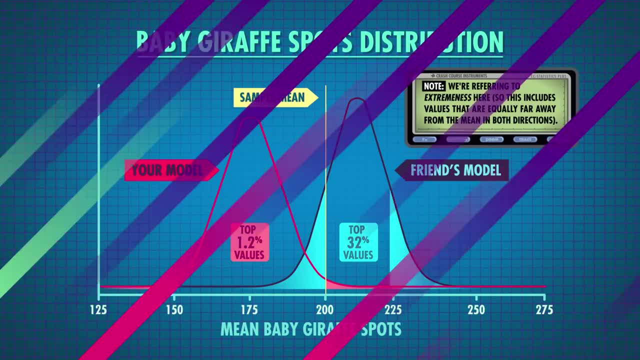 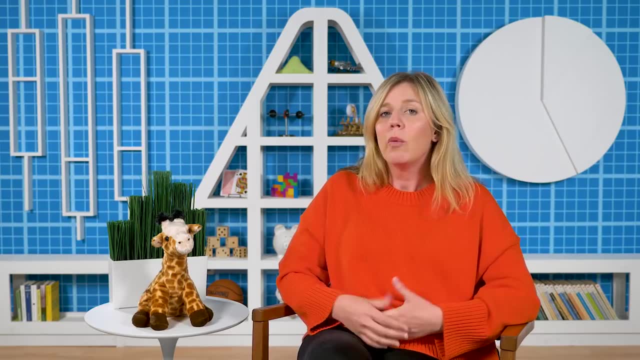 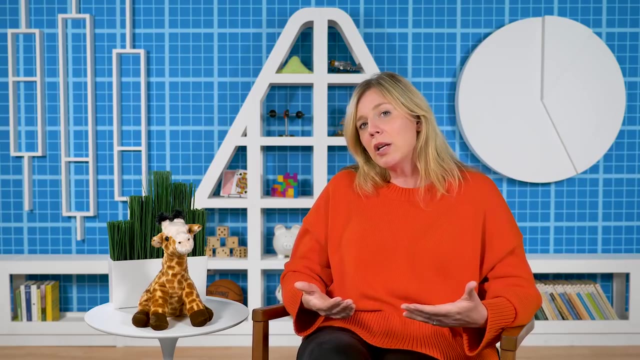 see sample means around 200, if you're right, But we don't always have predictions that are as specific as you and your friend's predictions about baby giraffe spots. We might have a more general hypothesis like that: the average number of baby giraffe spots is more than 200. But that's all you really. 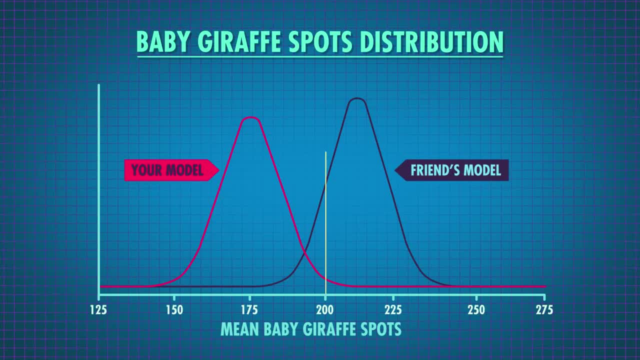 of sample means for your friend's model looks like this: Let's look at where our sample mean of 200 lies on both of these distributions. You can see that we're more likely to get a mean of 200 spots under your friend's hypothesis. 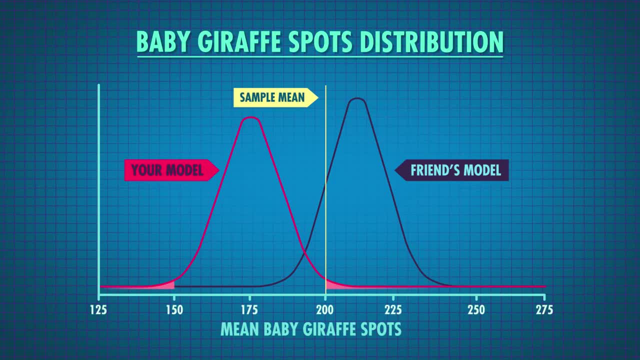 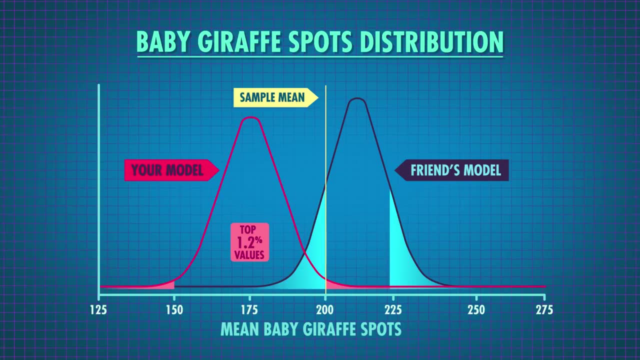 than yours. If your model were correct, a mean of 200 spots is pretty rare. It's in the top 1.2%, most extreme values we'd expect to see, Whereas in your friend's model a mean of 200 spots is only in the top 32%, which means it's pretty common that we'd 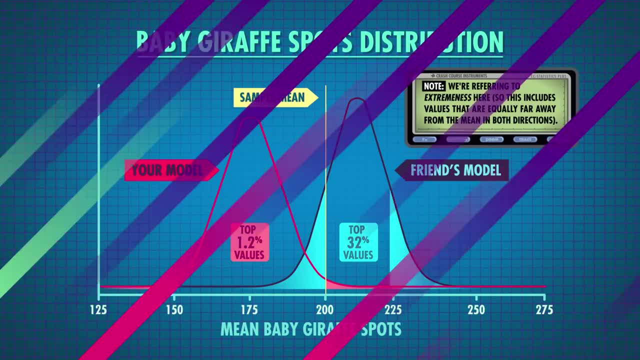 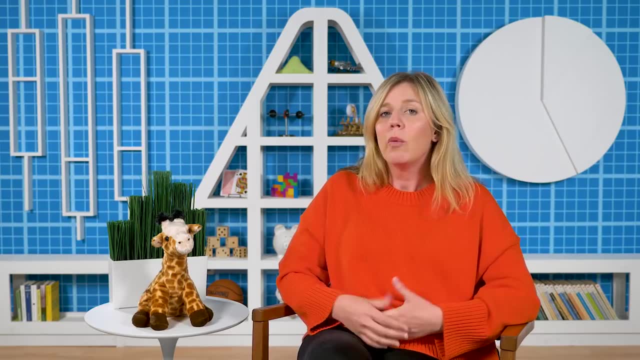 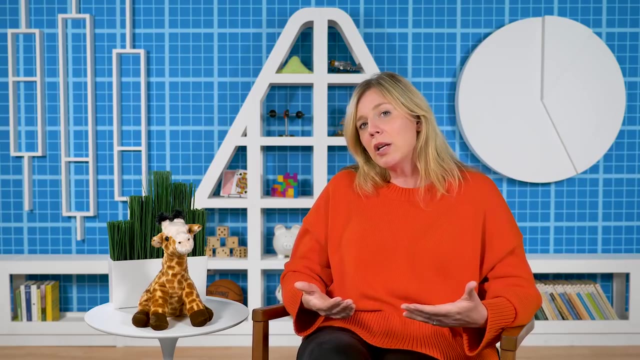 see sample means around 200, if you're right, But we don't always have predictions that are as specific as you and your friend's predictions about baby giraffe spots. We might have a more general hypothesis like that: the average number of baby giraffe spots is more than 200. But that's all you really. 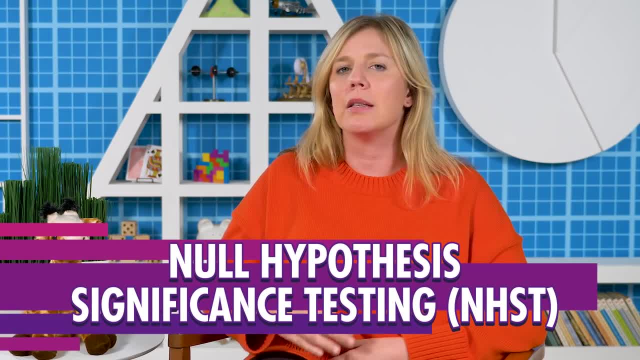 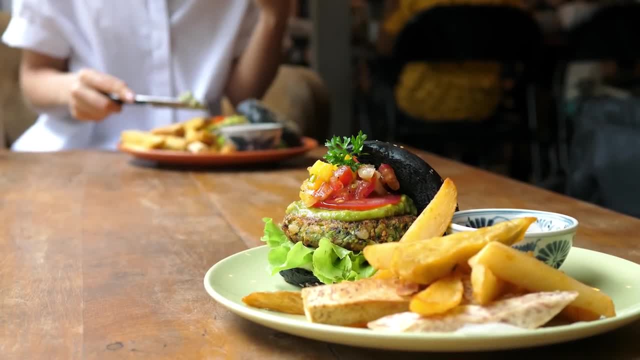 know. In situations like these, one common method of testing is null hypothesis significance testing. You have a hypothesis that people with a certain gene, we'll call it gene X- eat a different amount of calories than the general population. Null hypothesis testing is a very common method of testing. But if you're right then you're more likely to 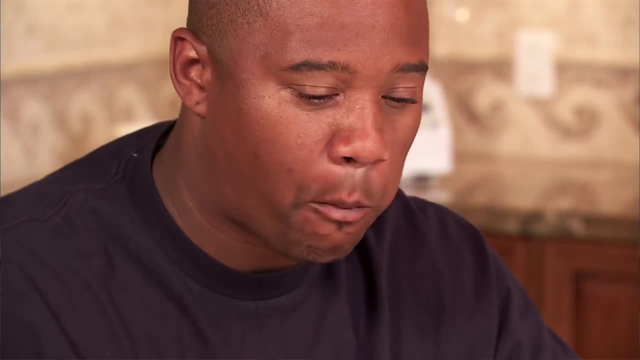 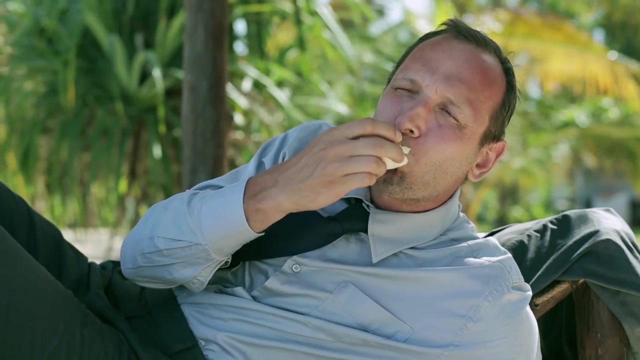 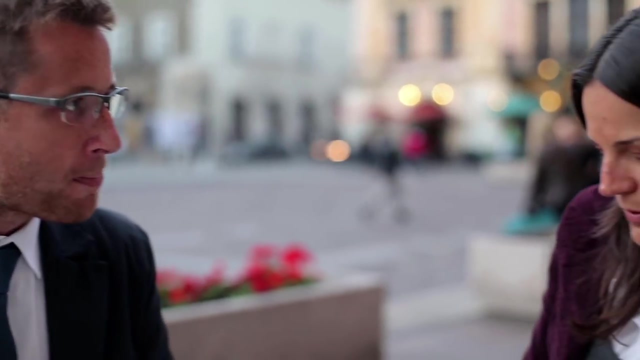 be wrong. Null hypothesis significance testing asks you to test a different hypothesis which says there's no difference or effect of this gene, And we'll see how well this null hypothesis predicts the data we've collected. In this case, the null hypothesis or null model is that the population mean caloric. 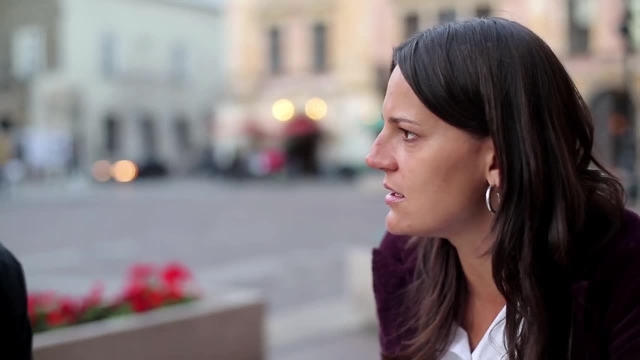 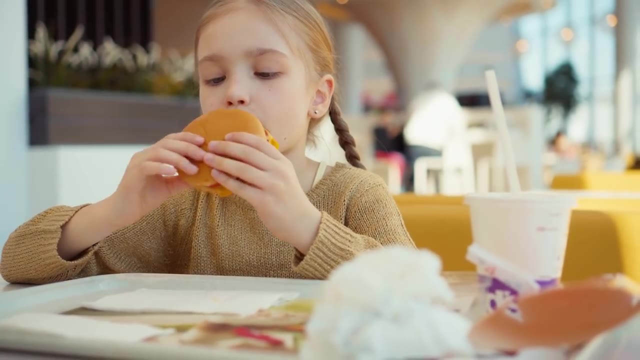 intake for people with gene X is actually 2300, the same as the regular population. If the null hypothesis is found to be infeasible, we can reject it. We can represent the gene X as a positive integer, And if the null hypothesis is found to be infeasible, we can represent the gene X as: 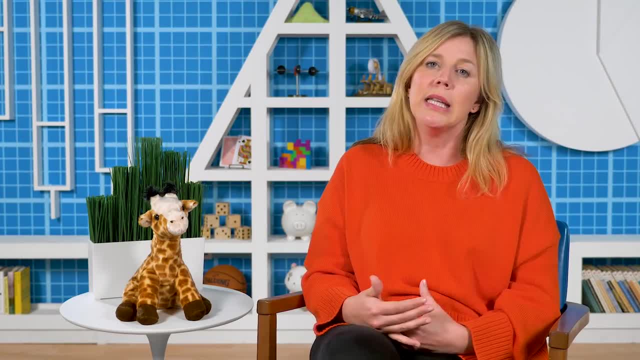 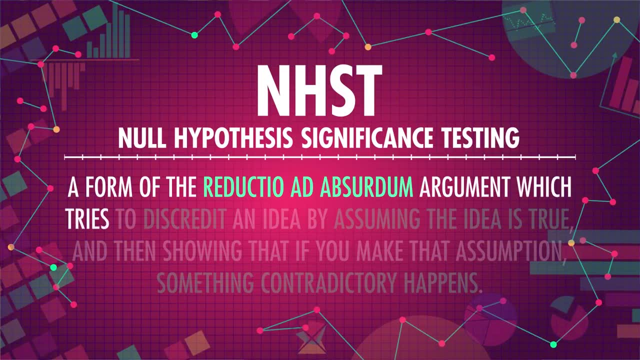 a positive integer. This might seem like a pretty roundabout way to test your theory that people with gene X eat differently And that's because it is Null hypothesis. significance testing is a form of the reductio ad absurdum argument, which tries to discredit an idea by assuming the idea is true and then showing that if 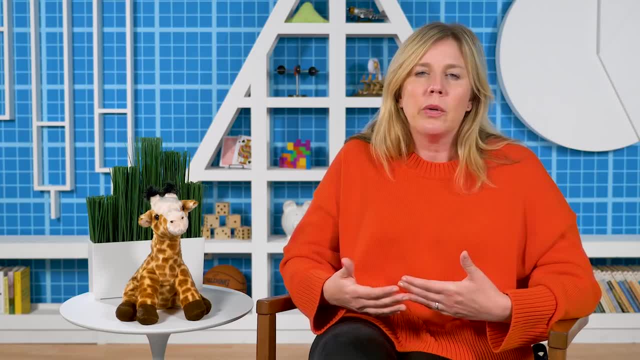 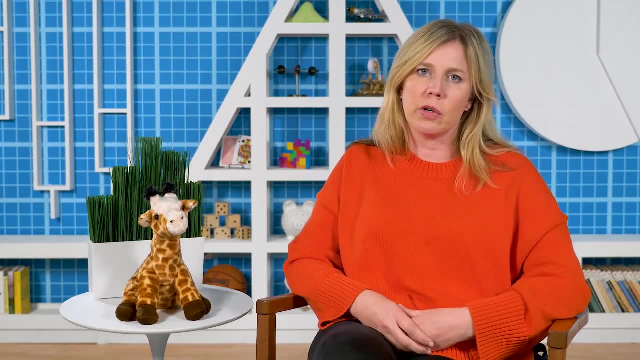 you make that assumption, something contradictory happens. For example, you can use reductio ad absurdum to show that there's no largest positive integer. Let's assume there IS a largest positive integer, We'll call it AB, for absurdly big. This means that there's. 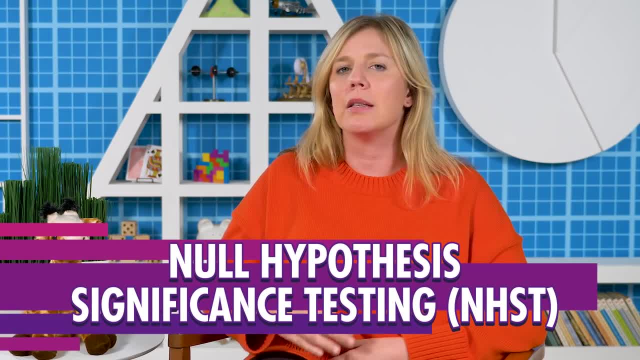 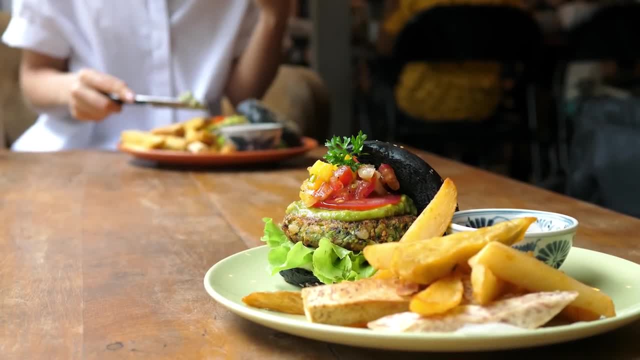 know. In situations like these, one common method of testing is null hypothesis significance testing. You have a hypothesis that people with a certain gene, we'll call it gene X- eat a different amount of calories than the general population. Null hypothesis testing is a very common method of testing. But if you're right then you're more likely to 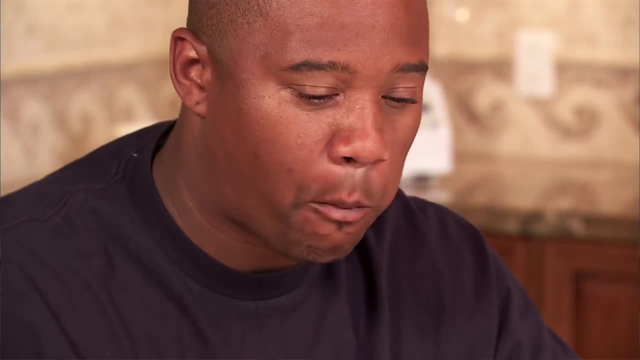 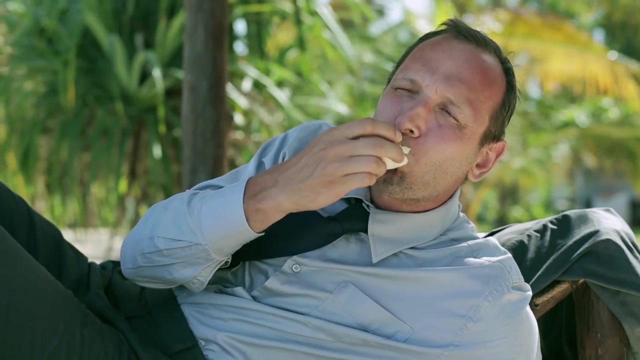 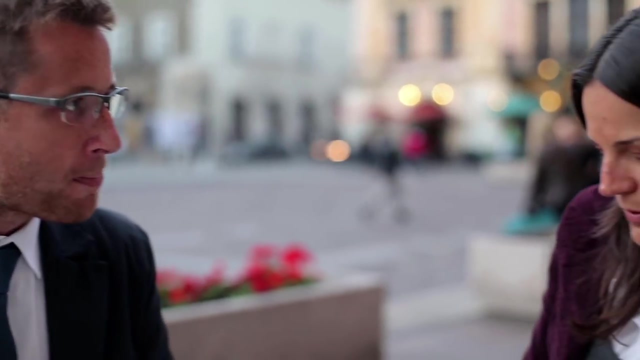 be wrong. Null hypothesis significance testing asks you to test a different hypothesis which says there's no difference or effect of this gene, And we'll see how well this null hypothesis predicts the data we've collected. In this case, the null hypothesis or null model is that the population mean caloric. 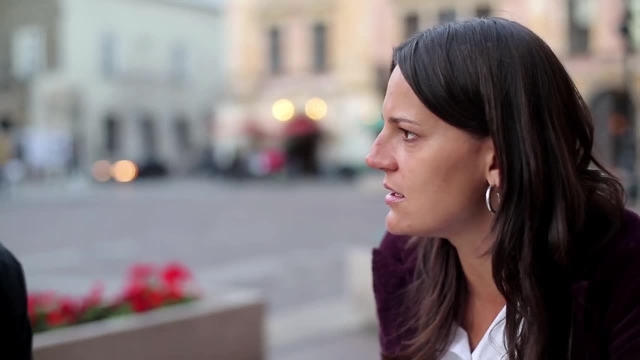 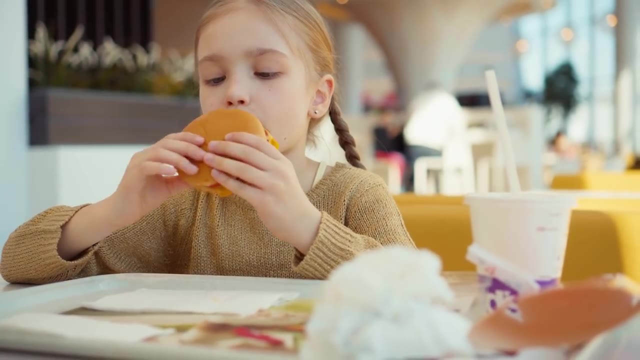 intake for people with gene X is actually 2300, the same as the regular population. If the null hypothesis is found to be infeasible, we can reject it. We can represent the gene X as a positive integer, And if the null hypothesis is found to be infeasible, we can represent the gene X as: 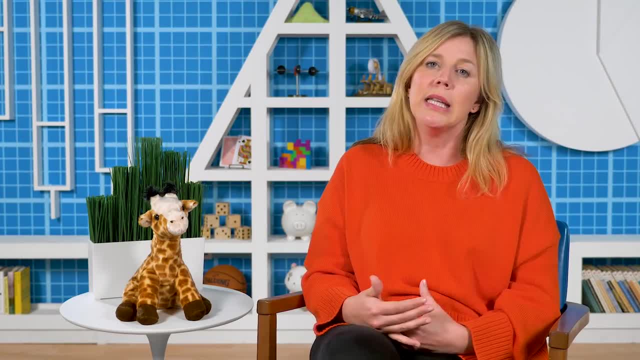 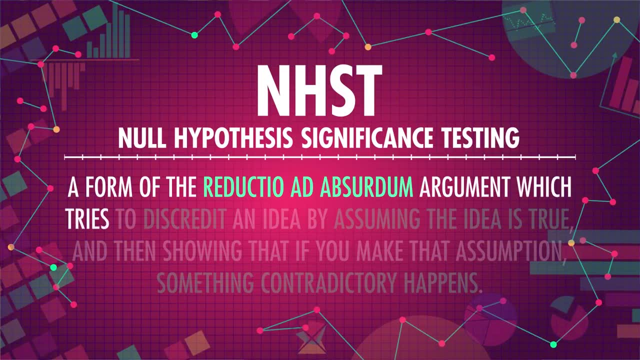 a positive integer. This might seem like a pretty roundabout way to test your theory that people with gene X eat differently And that's because it is Null hypothesis. significance testing is a form of the reductio ad absurdum argument, which tries to discredit an idea by assuming the idea is true and then showing that if 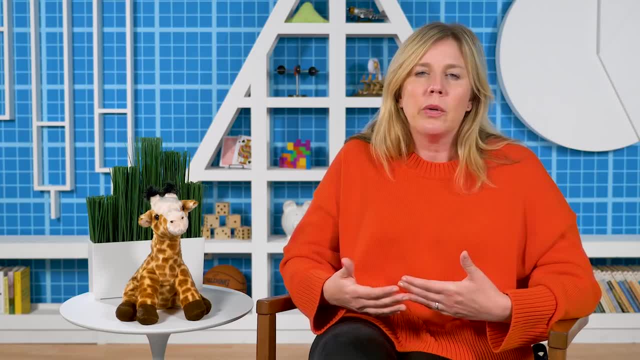 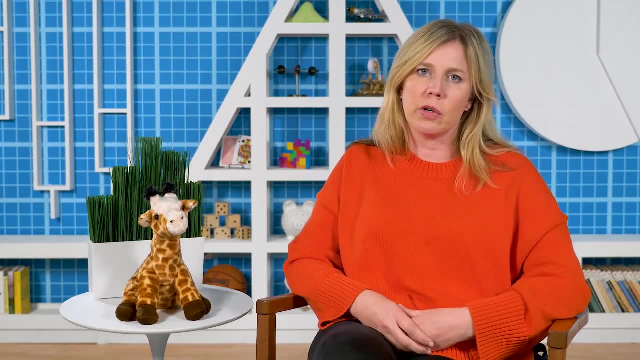 you make that assumption, something contradictory happens. For example, you can use reductio ad absurdum to show that there's no largest positive integer. Let's assume there IS a largest positive integer, We'll call it AB, for absurdly big. This means that there's. 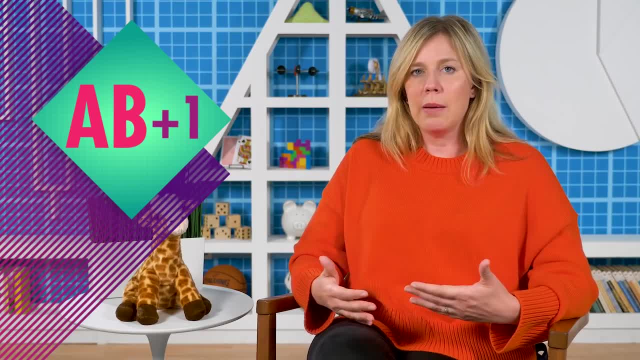 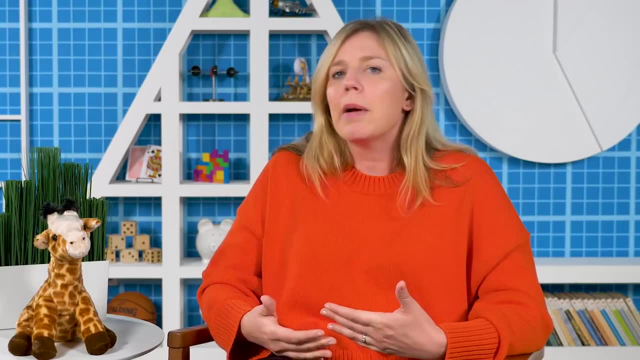 no largest positive integer. So let's assume there IS a largest positive integer. We'll call it AB, for absurdly big. Now we add 1 to AB, That would be a larger positive integer, which would be absurd since AB is the largest. Therefore, by reductio ad absurdum, there is no largest positive integer. 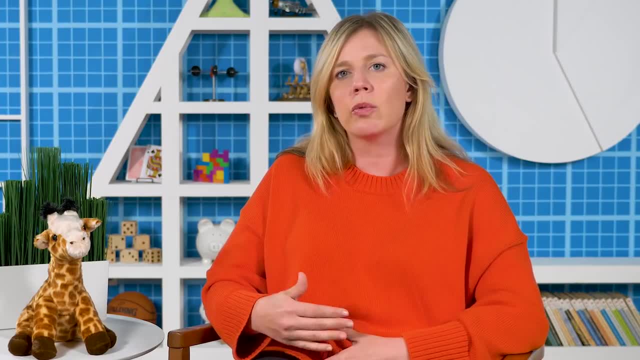 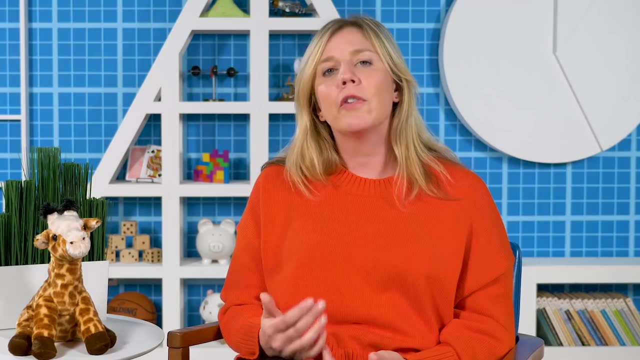 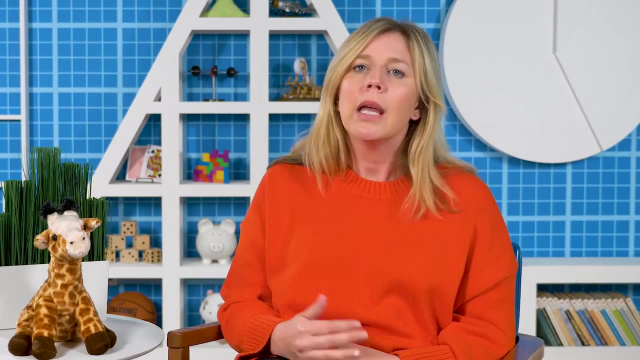 By the way, if this kind of argument sounds familiar, it might be because reductio ad absurdum is like proof by contradiction. Let's test the null hypothesis for our gene X case First. we assume that the mean number of calories eaten by people with gene X IS 2300, just like the regular population. If 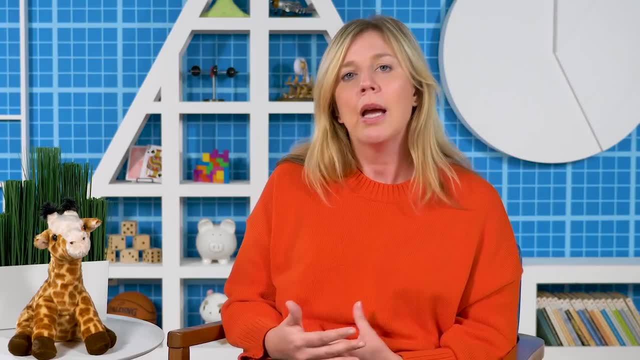 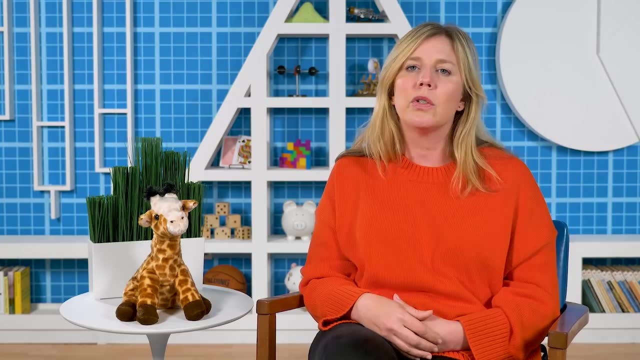 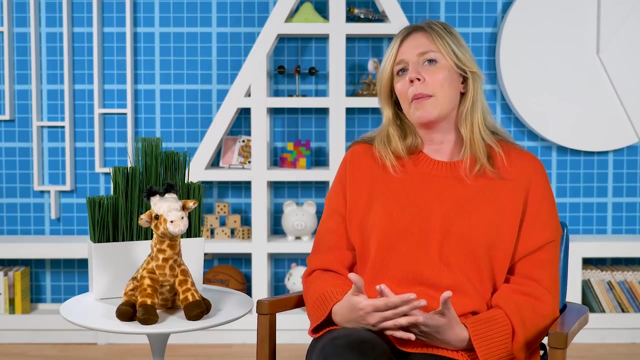 we can show that this assumption makes something absurd happen, then we can reject the idea that it's true. With data from 60 people with gene X, we see that the mean number of calories eaten was 2400, with a sample standard deviation of 500 calories. We have to ask how rare or absurd. 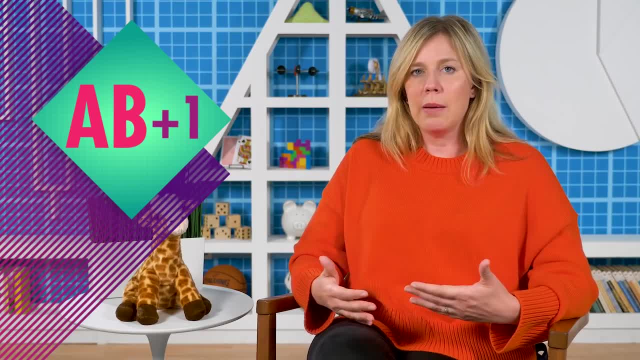 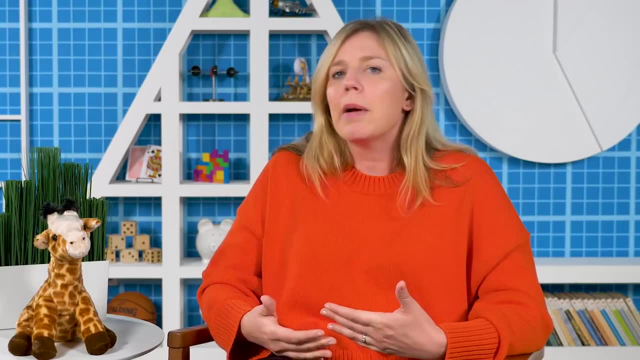 no largest positive integer. So let's assume there IS a largest positive integer. We'll call it AB, for absurdly big. Now we add 1 to AB, That would be a larger positive integer, which would be absurd since AB is the largest. Therefore, by reductio ad absurdum, there is no largest positive integer. 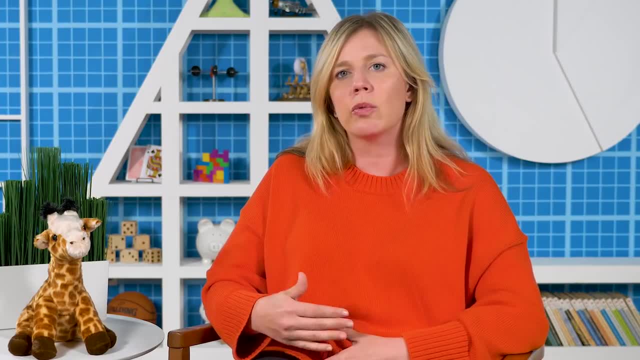 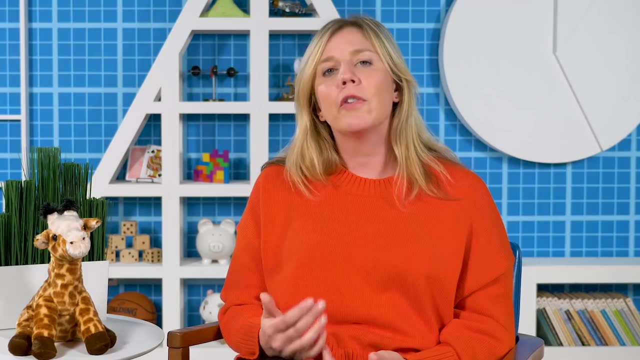 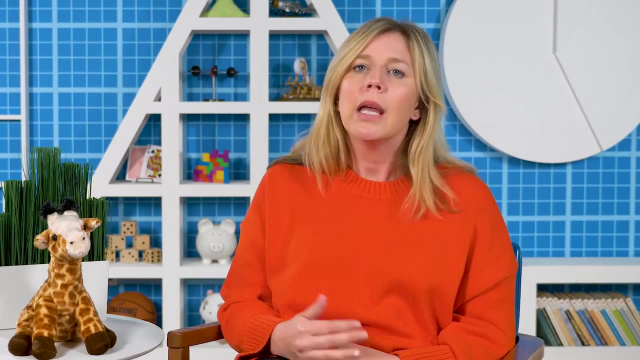 By the way, if this kind of argument sounds familiar, it might be because reductio ad absurdum is like proof by contradiction. Let's test the null hypothesis for our gene X case First. we assume that the mean number of calories eaten by people with gene X IS 2300, just like the regular population. If 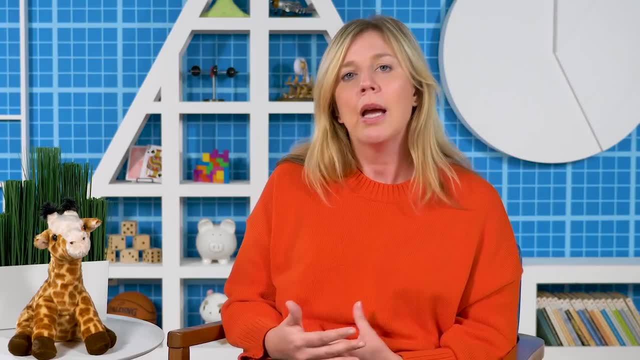 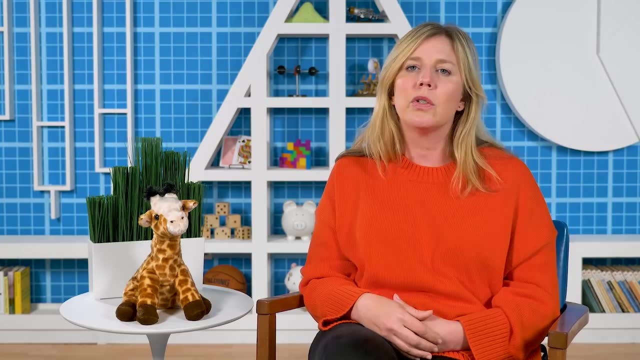 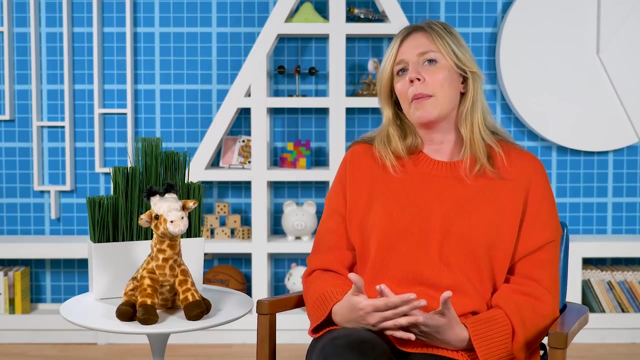 we can show that this assumption makes something absurd happen, then we can reject the idea that it's true. With data from 60 people with gene X, we see that the mean number of calories eaten was 2400, with a sample standard deviation of 500 calories. We have to ask how rare or absurd. 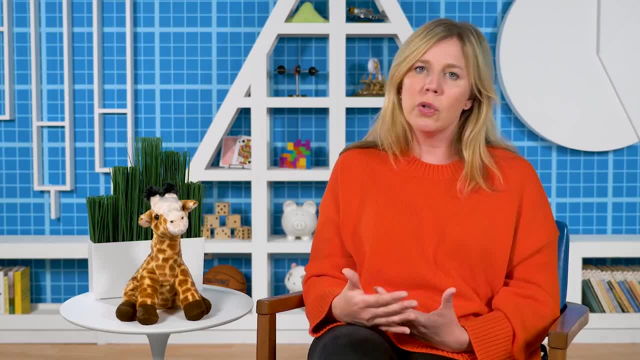 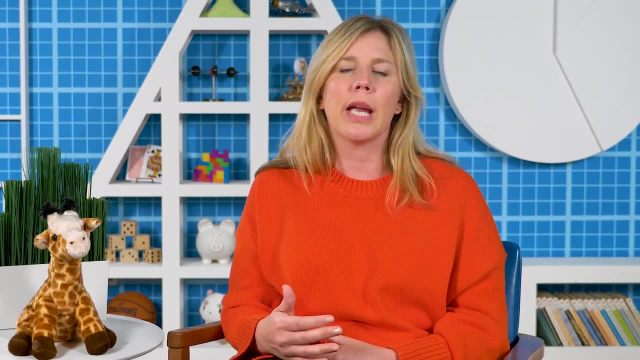 it would be to get a sample mean that is this far away from our assumed mean of 2300.. Essentially, we imagine that we take a random sample of 60 people with gene X, over and over and over again, And then we calculate the mean number of calories eaten by people with. 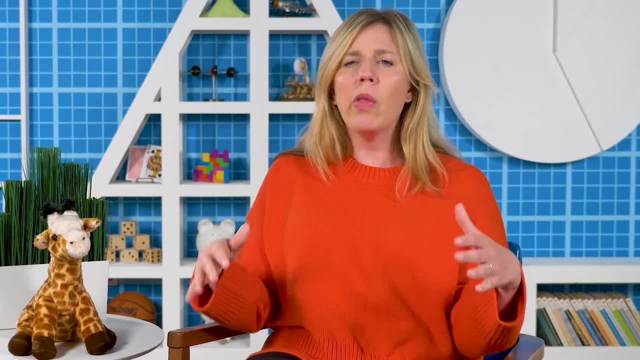 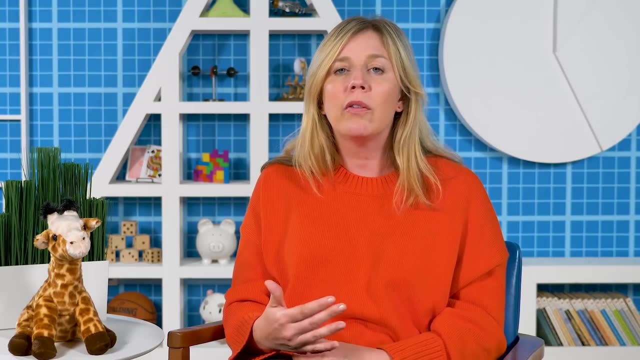 gene X. Then we ask: how many times out of all those experiments do we get a sample mean that's as far away from 2300 as our actual sample mean of 2400 is? Even if you haven't heard of the term null hypothesis significance testing, you might. 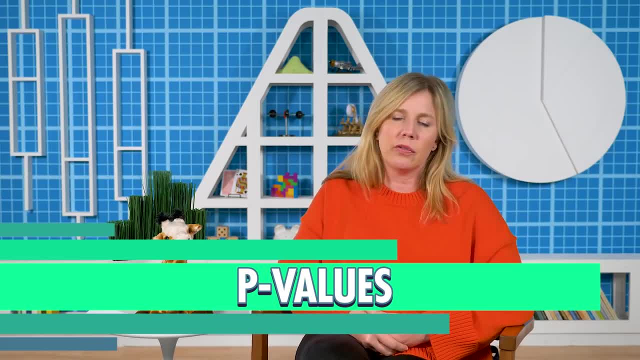 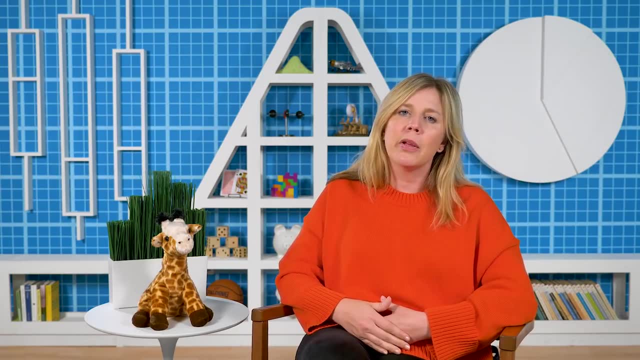 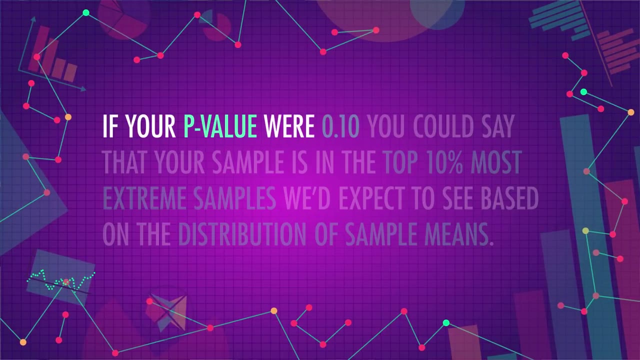 have heard of p-values, which have been covered everywhere, from academic journals to buzzfeed articles. A p-value answers the question of how rare your data is by telling you the probability of getting data that's as extreme as the data you observed. If your p-value were 0.10, you could say that your sample is in the top 10% most extreme. 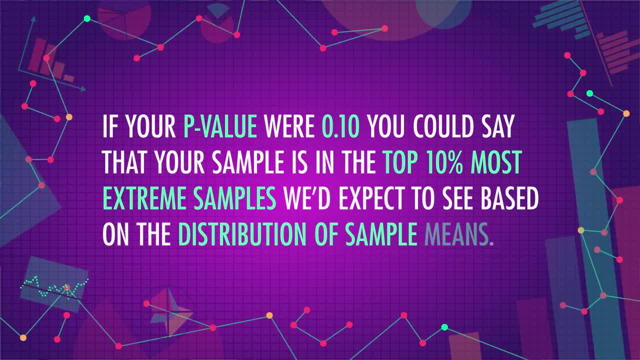 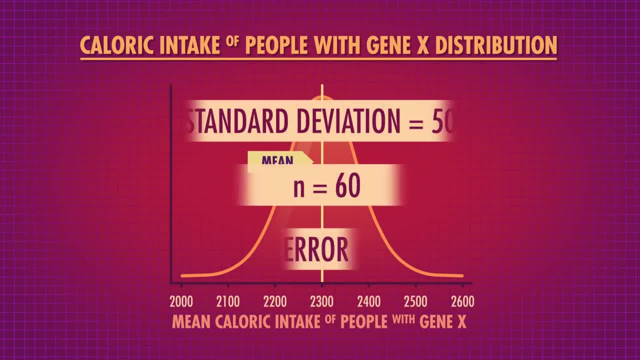 samples we'd expect to see, based on the distribution of sample means. If we assume that the null hypothesis is true and the mean caloric intake of people with gene x is 2300, with a standard deviation of 500 calories, the distribution of sample means. 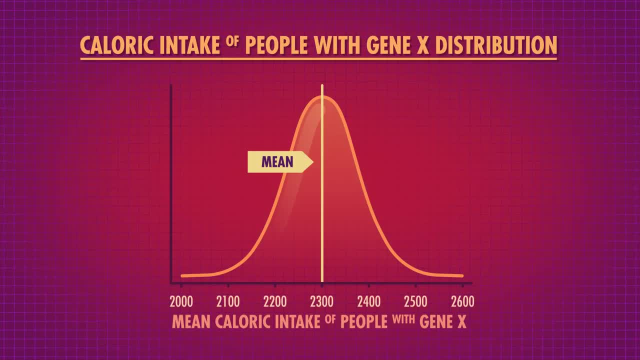 will look like this and tells us which means we expect to see and how often we expect to see each of them. Sample means around 2300 are most common, so you can see that there's a positive number of people with gene X. that's approximately less than 2300.. This is the 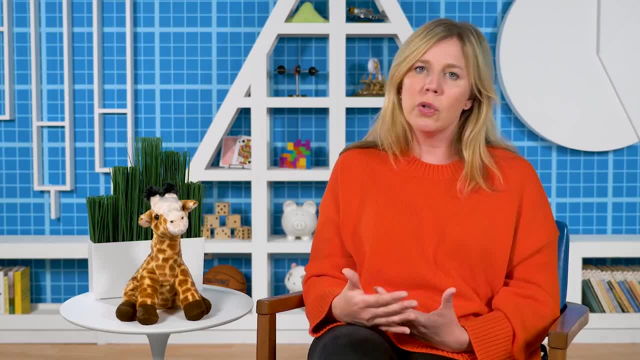 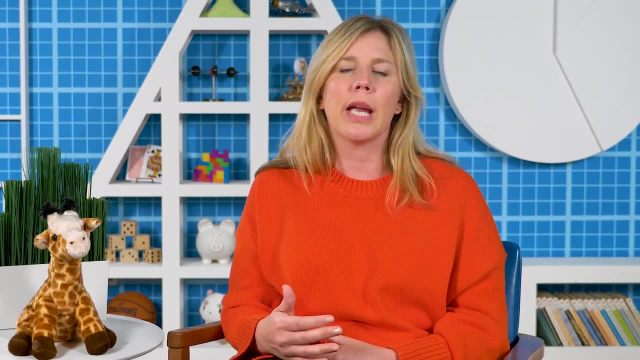 it would be to get a sample mean that is this far away from our assumed mean of 2300.. Essentially, we imagine that we take a random sample of 60 people with gene X, over and over and over again, And then we calculate the mean number of calories eaten by people with. 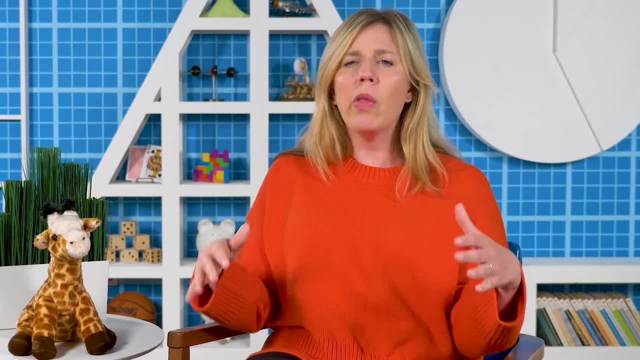 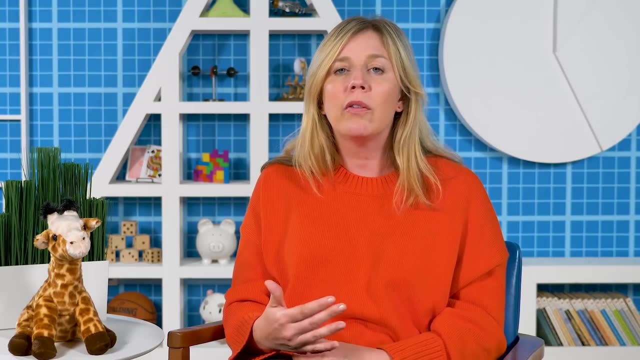 gene X. Then we ask: how many times out of all those experiments do we get a sample mean that's as far away from 2300 as our actual sample mean of 2400 is? Even if you haven't heard of the term null hypothesis significance testing, you might. 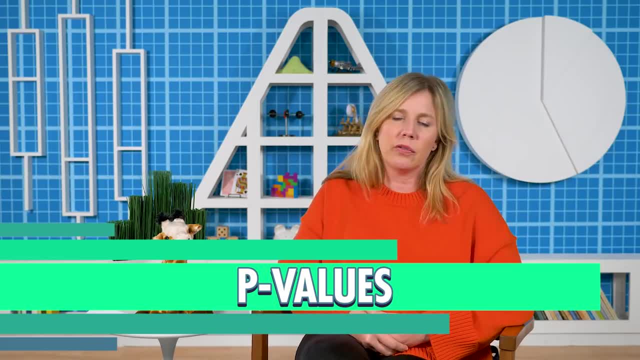 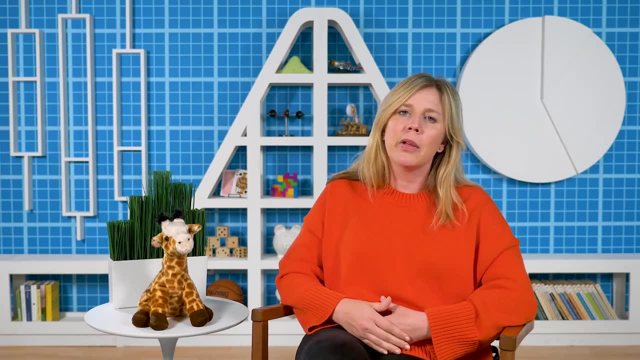 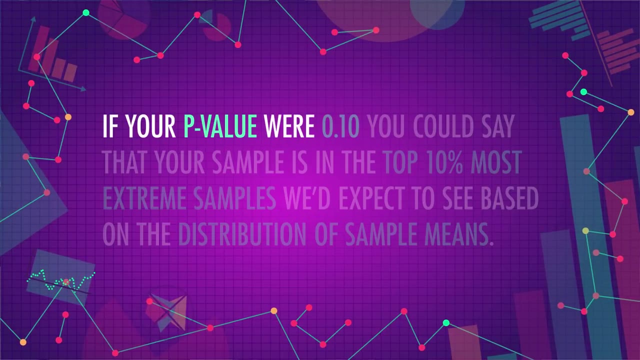 have heard of p-values, which have been covered everywhere, from academic journals to buzzfeed articles. A p-value answers the question of how rare your data is by telling you the probability of getting data that's as extreme as the data you observed. If your p-value were .10, you could say that your sample is in the top 10% most extreme. 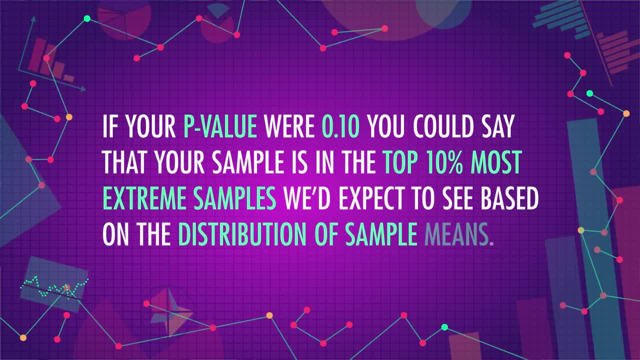 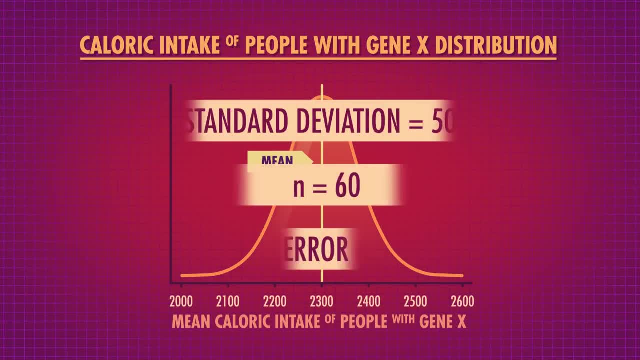 samples we'd expect to see, based on the distribution of sample means. If we assume that the null hypothesis is true and the mean caloric intake of people with gene X is 2300, with a standard deviation of 500 calories, the distribution of sample. 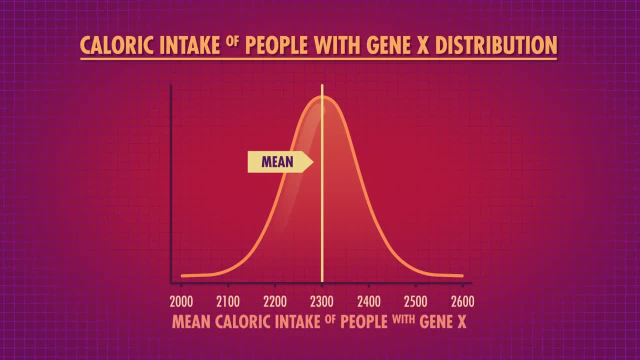 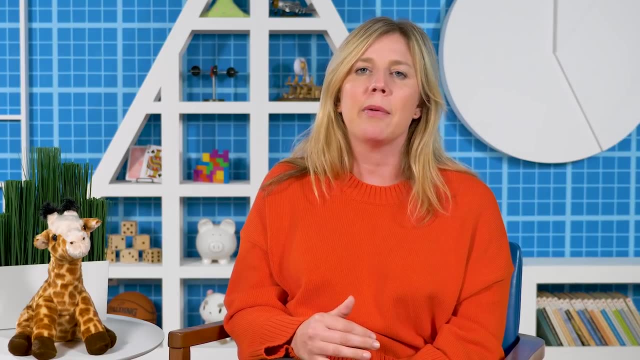 means will look like this and tells us which means we expect to see and how often we expect to see each of them. Sample means- around 2300- are most common. The most common means are common, but we'll also often see sample means a little bit further away. 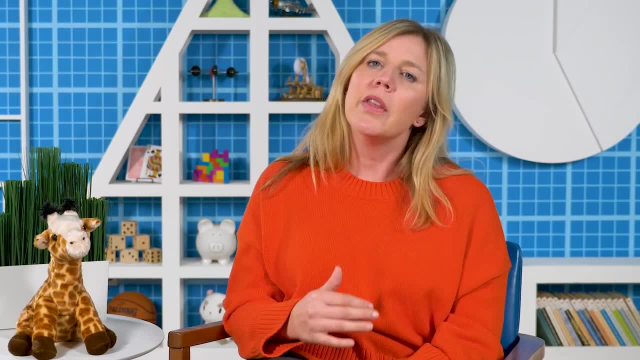 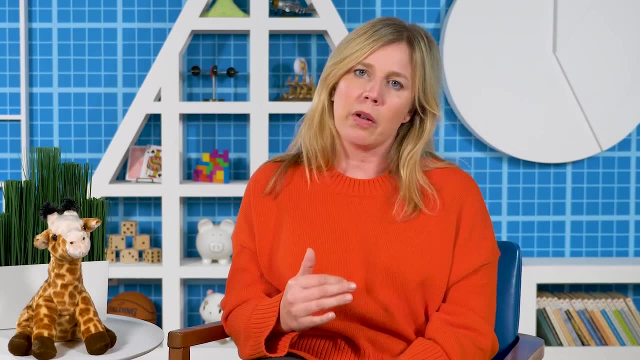 We can use this distribution to calculate our p-value. This is similar to how we compared the likelihood of 200 giraffe spots in you and your friends models, but with only one model this time. Here's our sample mean of 2400 on this graph. 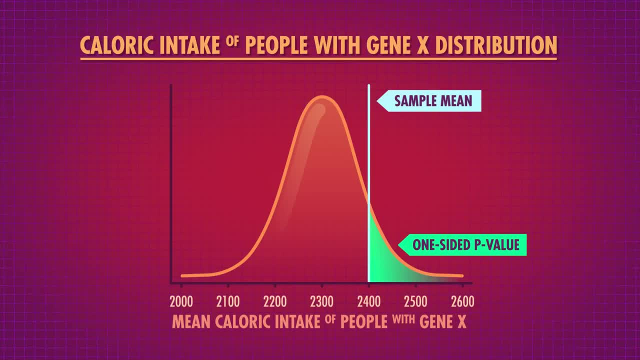 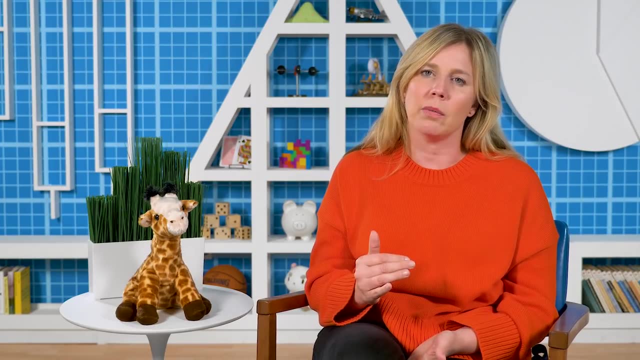 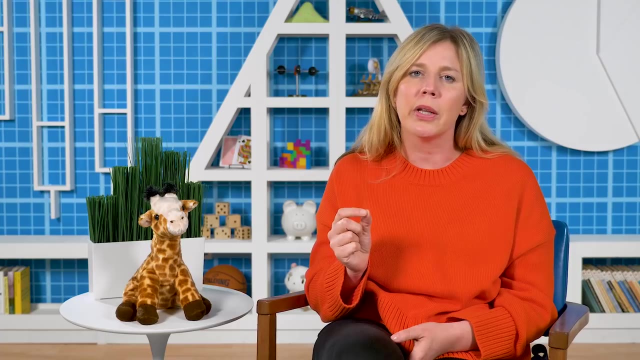 Only about 8.99% of the possible sample means are higher than 2400, so it's not that unlikely that we get a sample mean that's this high if the true population mean was 2300 calories. This is called a one-sided p-value since it only tells us the probability of getting. 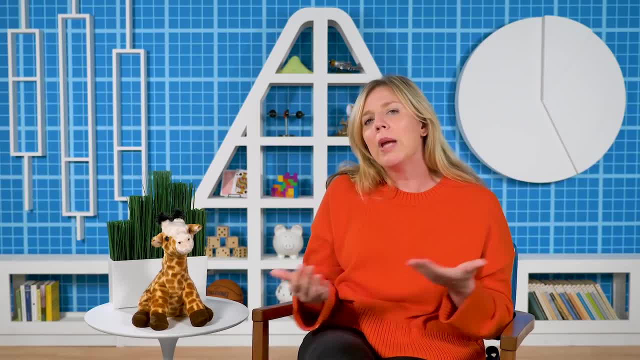 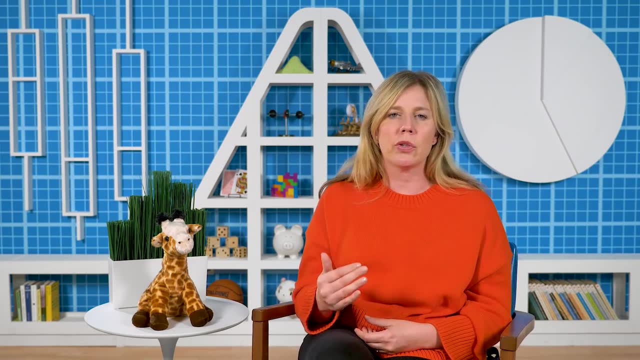 a sample mean that's higher than 2400.. Often when we ask scientific questions like does this medicine have a different level of efficacy than the existing treatment, we don't know which direction the effect will be in. The new medicine might be better or it might be worse. 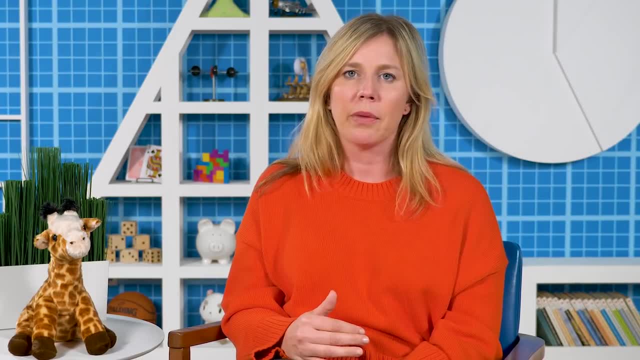 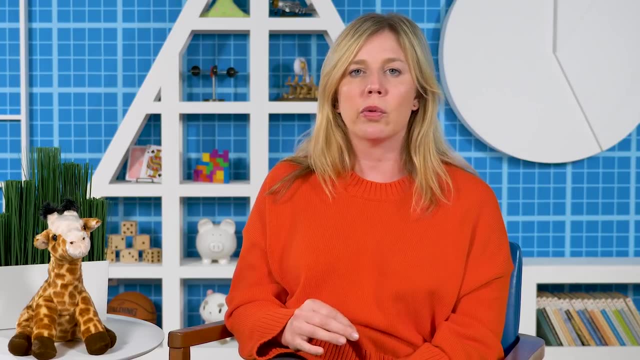 common, but we'll also often see sample means a little bit further away. We can use this distribution to calculate our p-value. This is similar to how we compared the likelihood of 200 giraffe spots in you and your friend's models, but with only one model this time. Here's our 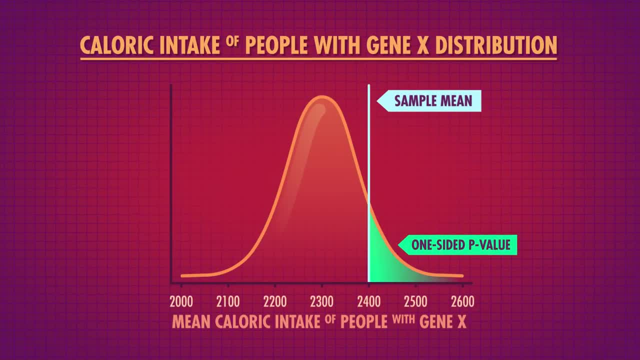 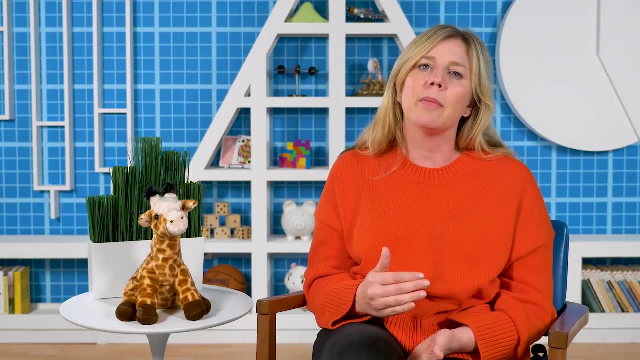 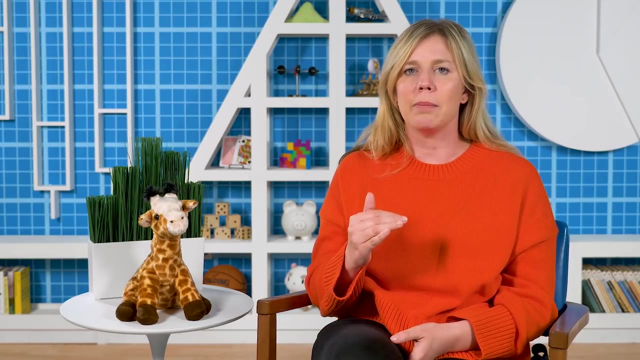 sample mean of 2400. on this graph, Only about 8.99% of the possible sample means are higher than 2400, so it's not that unlikely that we'd get a sample mean that's this high if the true population mean was 2300 calories. This is called a one-sided p-value, since it only tells us the 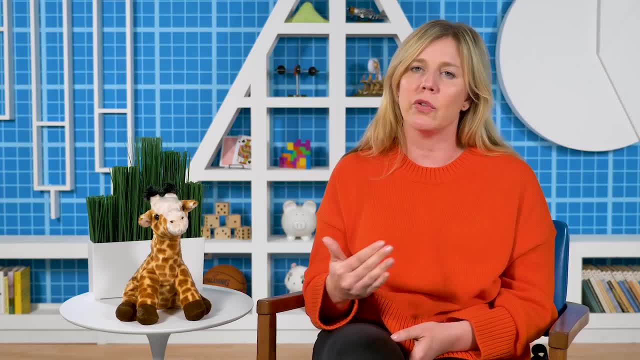 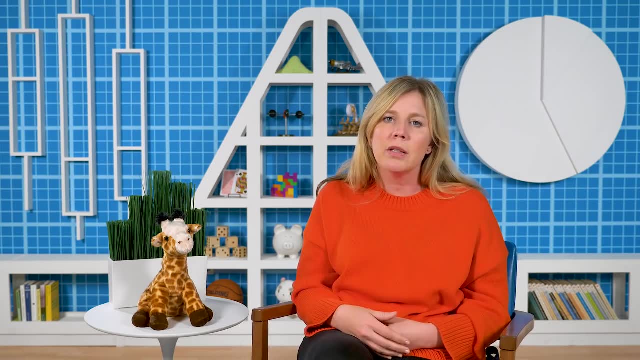 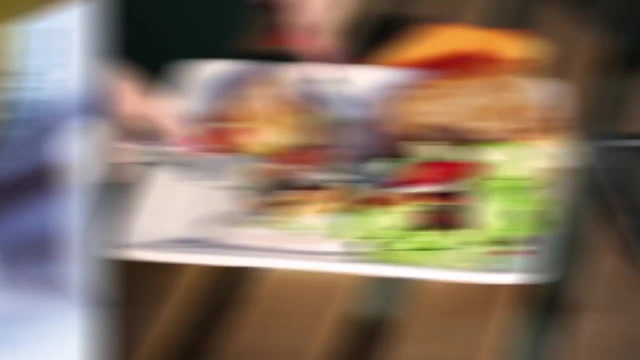 probability of getting a sample mean that's higher than 2400.. Often, when we ask scientific questions like does this medicine have a different level of efficacy than the existing treatment, we don't know which direction the effect will be in. The new medicine might be better or it might be worse. 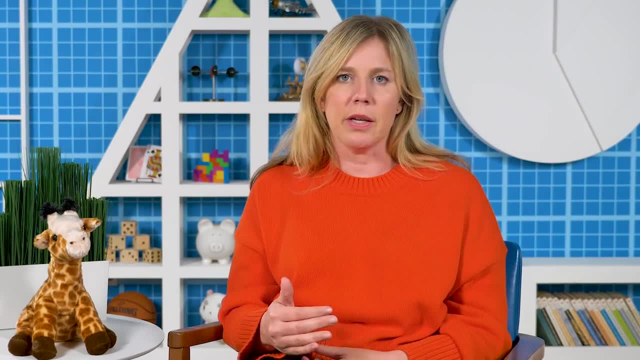 Gene Xers might eat more or they might eat less. Because of this and a few other reasons we'll talk about in the next video. we're going to talk about the effect of the new medicine Later in the series. p-values are often two-sided, meaning that we look at how far away a value is. 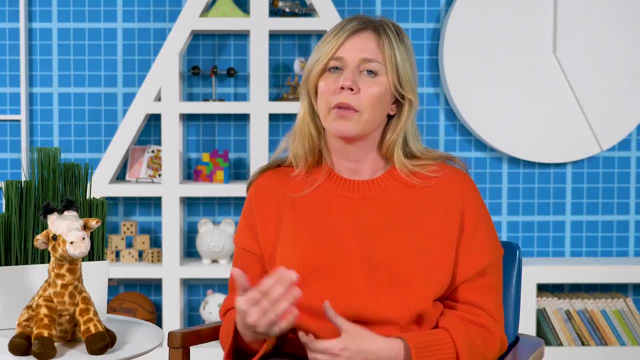 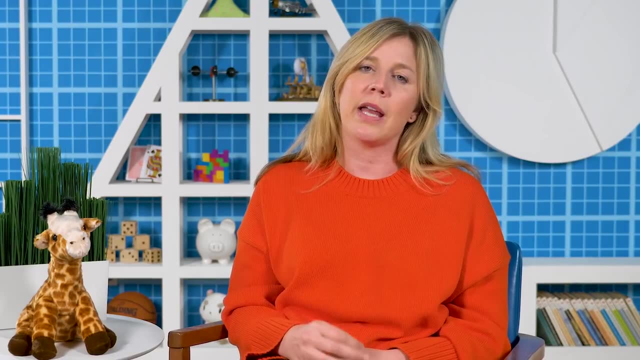 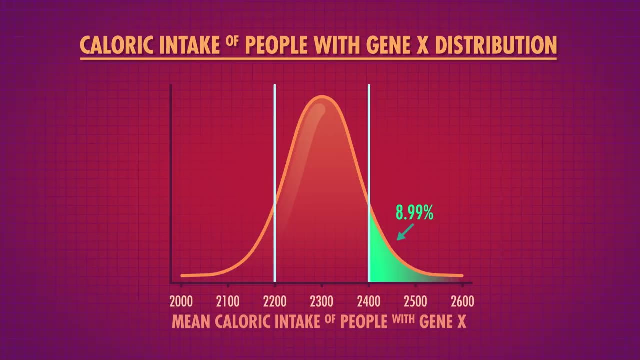 from the mean, regardless of if it's higher or lower. This allows us to reject the null hypothesis if our value is significantly higher than the mean or if the value is significantly lower than the mean, Because the distribution of sample means is symmetrical. if 9% of the samples of caloric 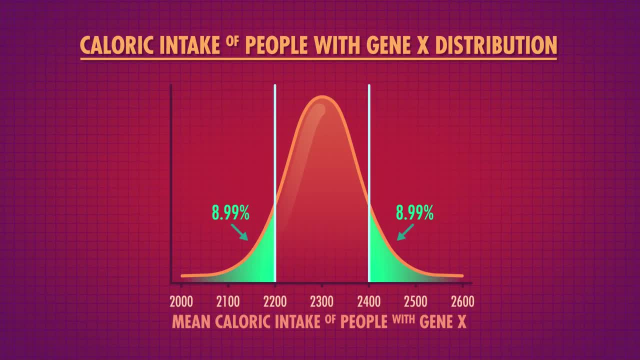 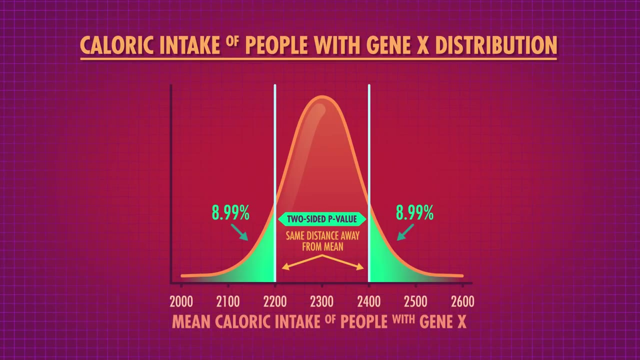 intake are higher than a mean of 2400, about 18% of sample means for calories would be as far away or further from the population mean than 2400 is in either direction. In other words, a two-sided p-value is a measure of how extreme your sample mean is. 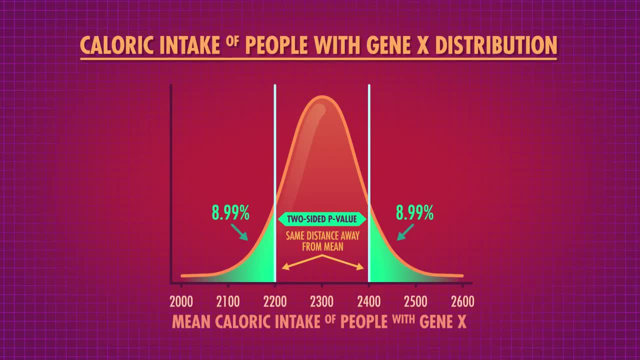 because it tells you how often you'll get a value that's as or more extreme than the one you got. The smaller your p-value is, the more rare it would be to get your sample just by random chance alone. if the null is true. 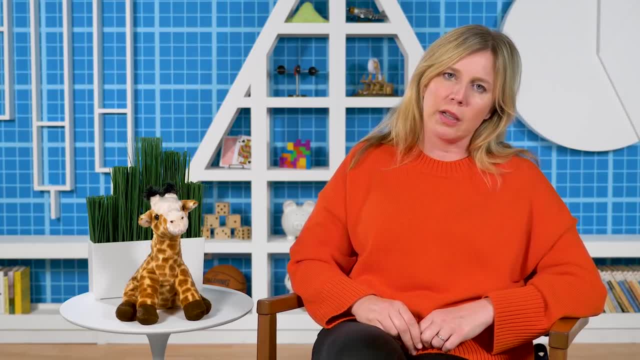 In our example we learned that if we assume that there's no effect of gene X on caloric intake, then there would be an 8% chance that the sample would be lower than 2400.. And then there would be an 18% chance that we'd see a sample like this. 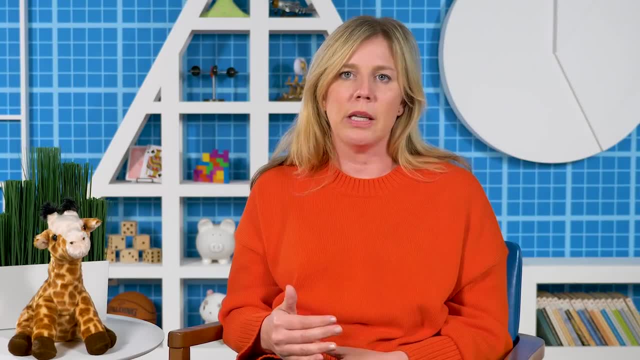 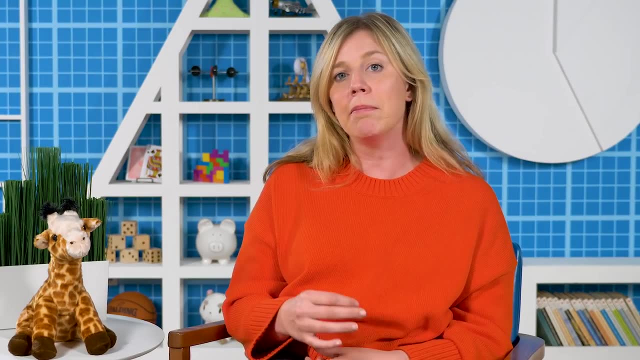 Gene Xers might eat more Or they might eat less. Because of this and a few other reasons we'll talk about later in the series, p-values are often two-sided, meaning that we look at how far away a value is from the mean regardless. 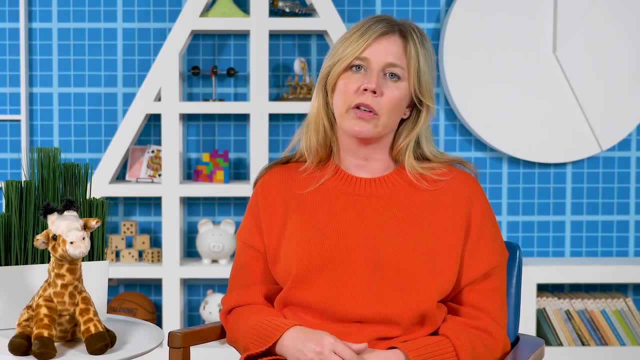 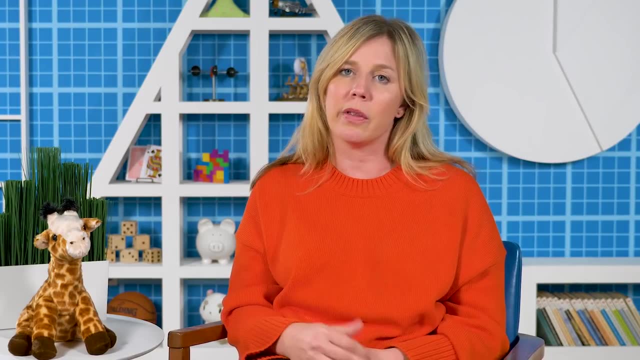 of if it's higher or lower. This allows us to reject the null hypothesis if our value is significantly higher than the mean or if the value is significantly lower than the mean, Because the distribution of sample means is symmetrical. if 9% of the samples of caloric 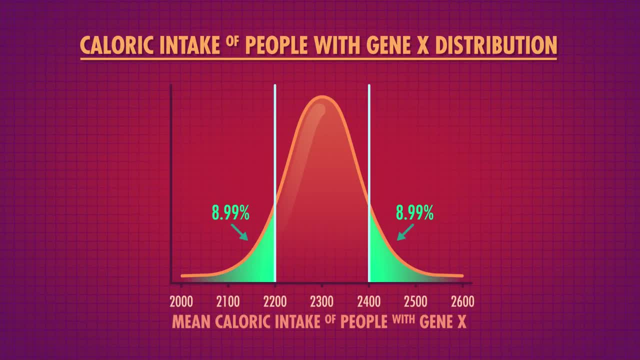 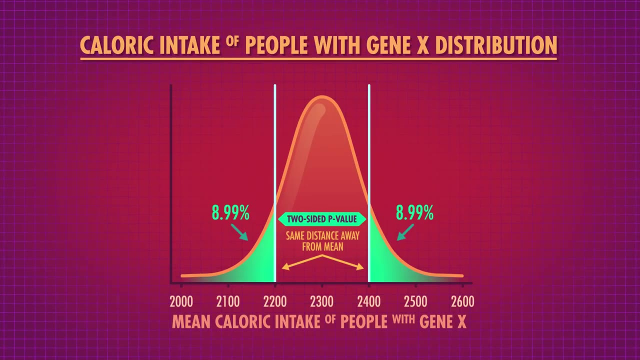 intake are higher than a mean of 2400, about 18% of the sample means are higher than a mean of 2400.. In other words, a two-sided p-value is a measure of how extreme your sample mean is, because it tells you how often you'll get a value that's as or more extreme than the one you 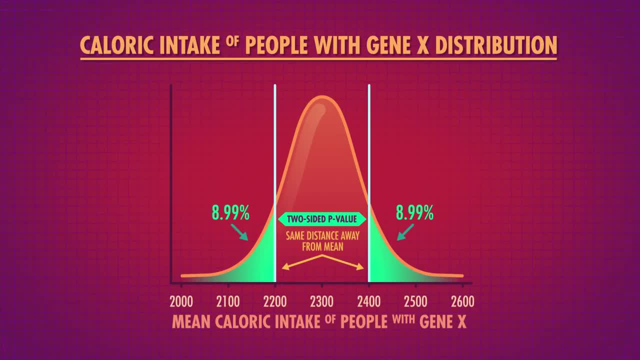 got. The smaller your p-value is, the more rare it would be to get your sample just by random chance alone. if the null is true In our example, we learned that if we assume that there's no effect on the sample, then 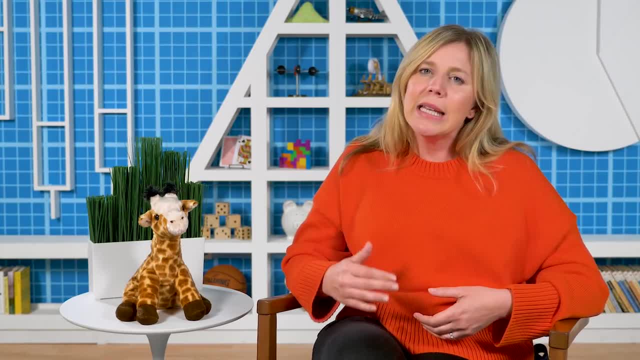 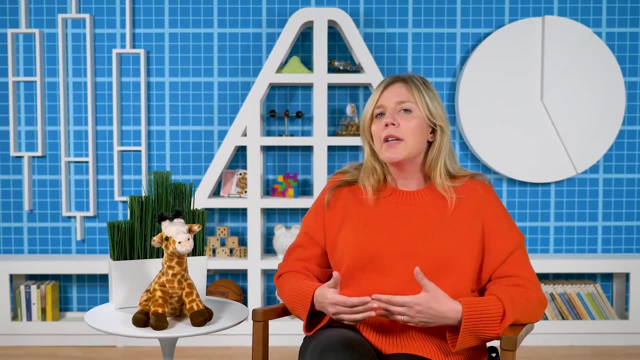 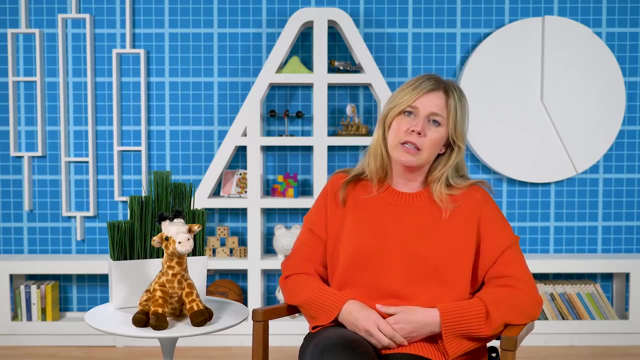 there would be an 18% chance that we'd see a sample like this just because of the random variation of samples. To finish our attempt at reductio ad absurdum, we have to decide whether this sample is absurd or extreme enough to lead us to believe that this sample probably isn't from the null. 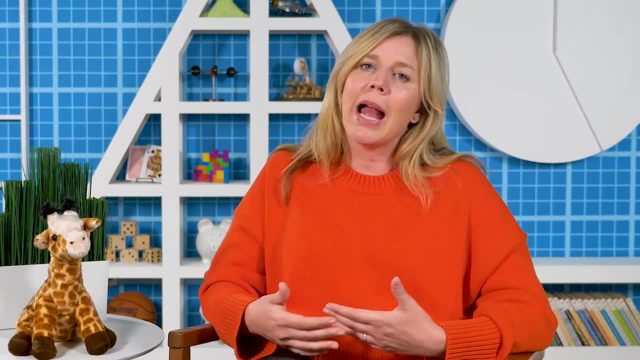 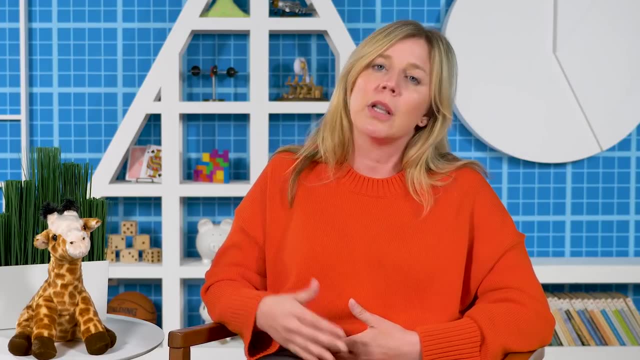 distribution, But that decision isn't always an easy one to make. It's not clear how rare or absurd a sample needs to be. before I decide to reject the idea that the sample is like this, It's clear that the sample was taken from a population that has the null distribution. 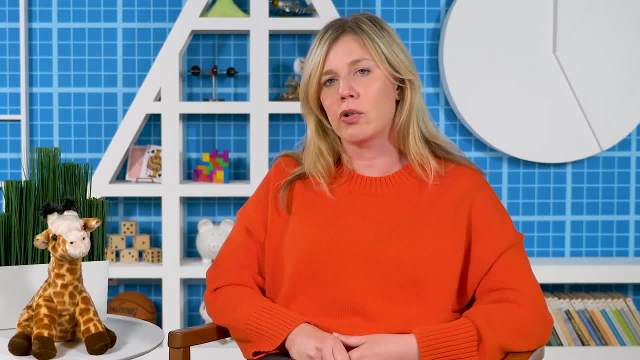 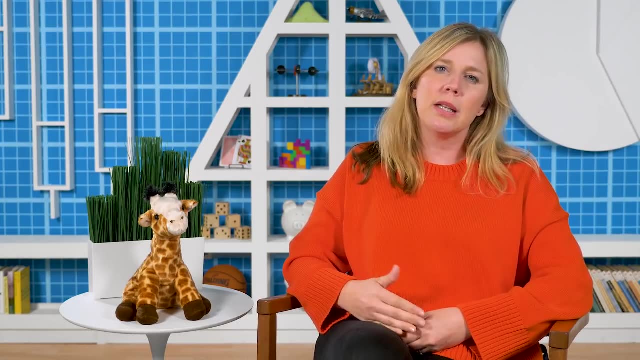 especially since we don't have another distribution to compare it to, like we did with the giraffes. Our p-value of 0.18 tells us that if we took a sample like this over and over and over- about one out of every five times- we'd get a sample with a mean caloric intake that's. 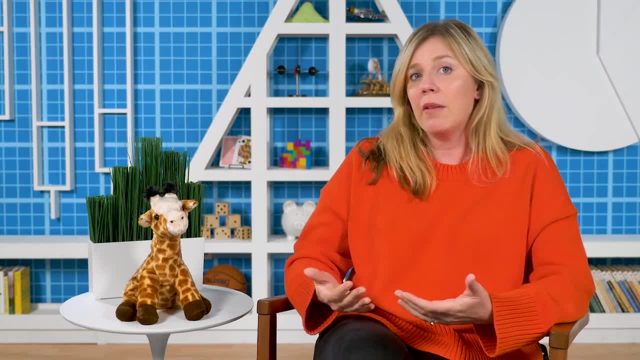 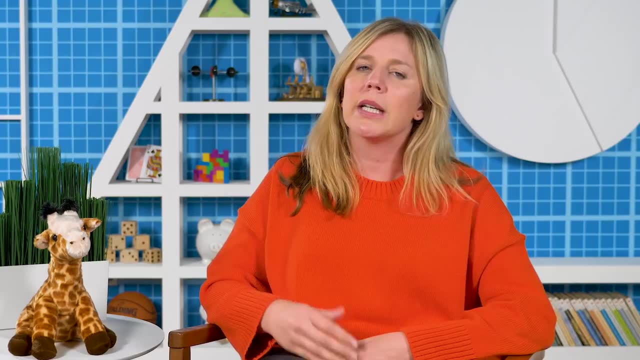 further from the mean than 2400 calories. is One in five's not bad, but a one in twenty chance might be better and a one in one hundred chance better than that. Some statisticians see a p-value as a continuous measure of evidence. 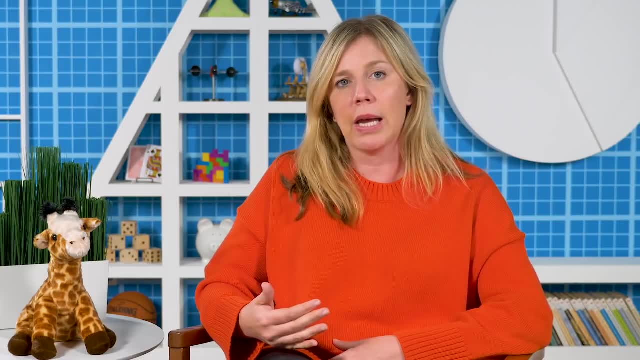 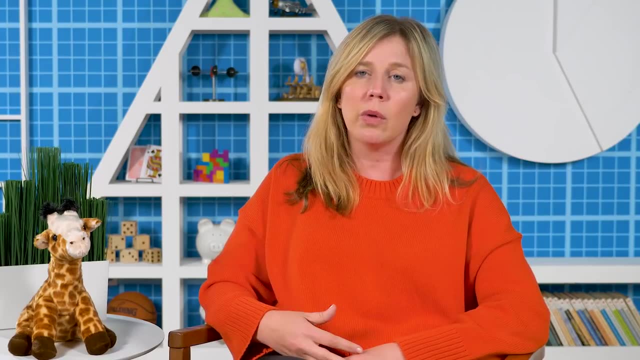 A p-value of 0.18, like ours might be considered pretty weak evidence that our sample isn't taken from the null distribution, but it's better than a 0.19, which is in turn better than a 0.20, and on and on. 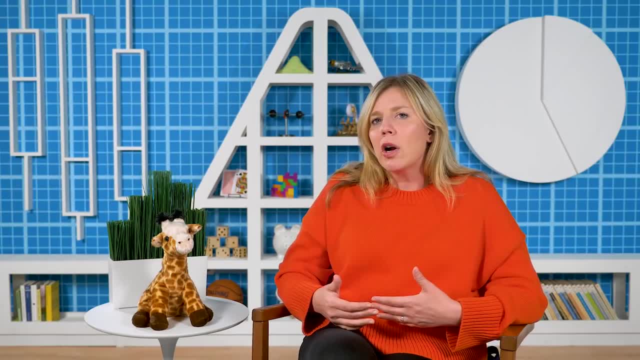 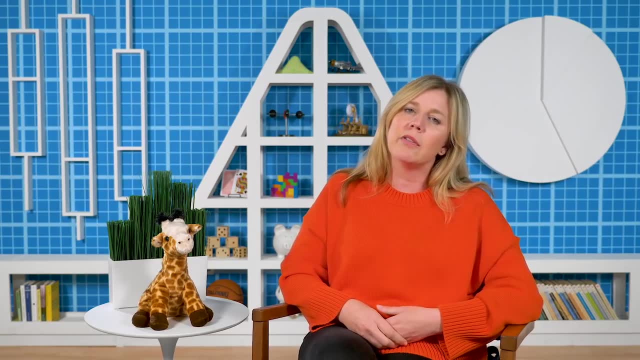 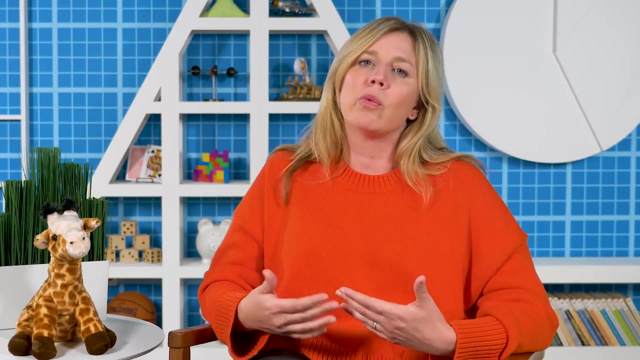 just because of the random variation of samples. To finish our attempt at reductio ad absurdum, we have to decide whether this sample is absurd or extreme enough to lead us to believe that this sample probably isn't from the null distribution. But that decision isn't always an easy one to make. It's not clear how rare or absurd 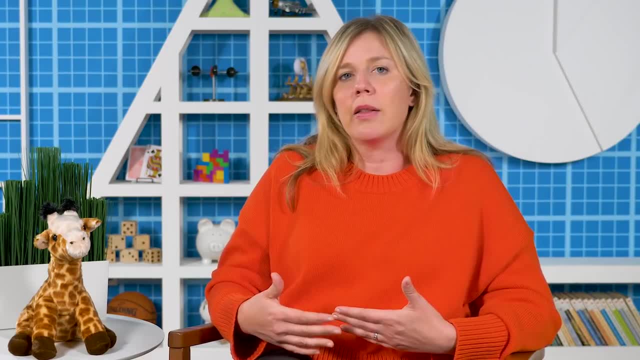 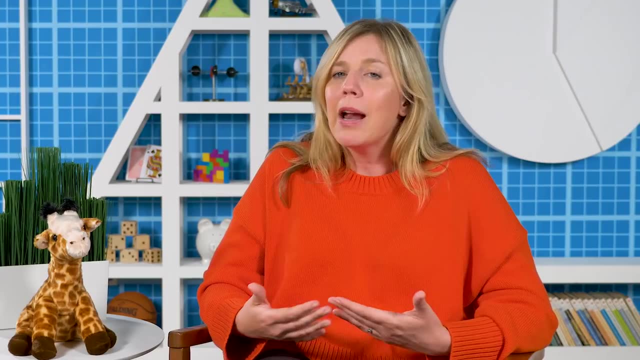 a sample needs to be before I decide to reject the idea that this sample was taken from a population that has the null distribution, Especially since we don't have another distribution to compare it to, like we did with the giraffes. Our p-value of 0.18 tells us that if we took a sample like this over and over and over, 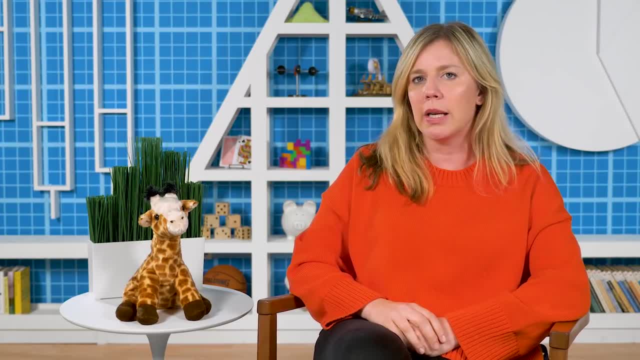 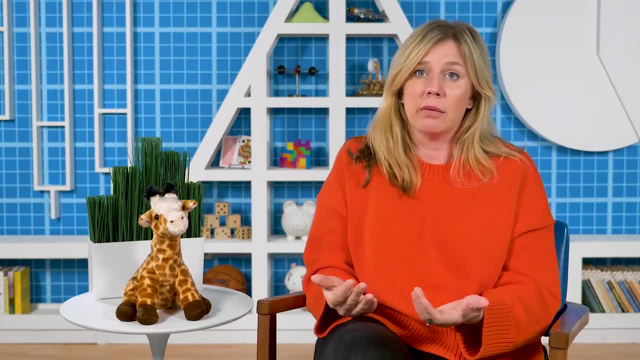 about 1 out of every 5 times. we'd get a sample with a mean caloric intake that's further from the mean than 2400 calories. is 1 in 5's not bad, but a 1 in 20 chance might be better. 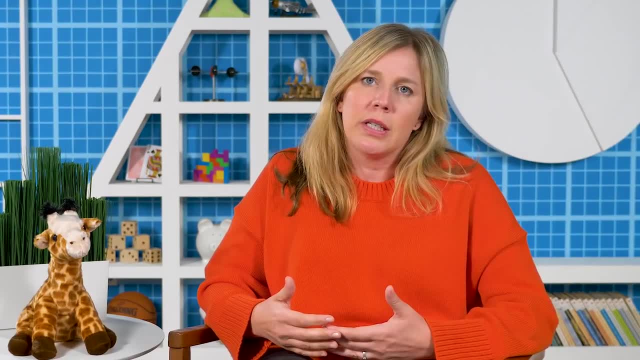 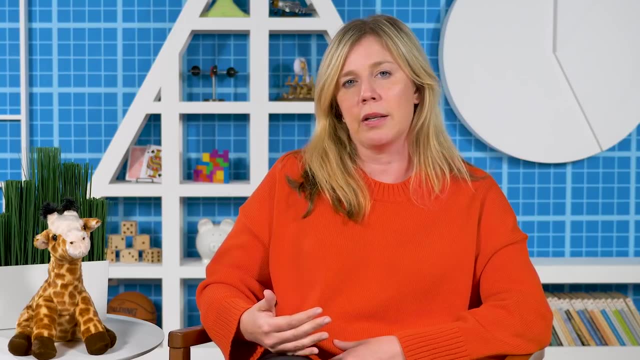 and a 1 in 100 chance better than that. Some statisticians see a p-value as a continuous measure of evidence. A p-value of 0.18, like ours, might be considered pretty good. There's pretty weak evidence that our sample isn't taken from the null distribution. 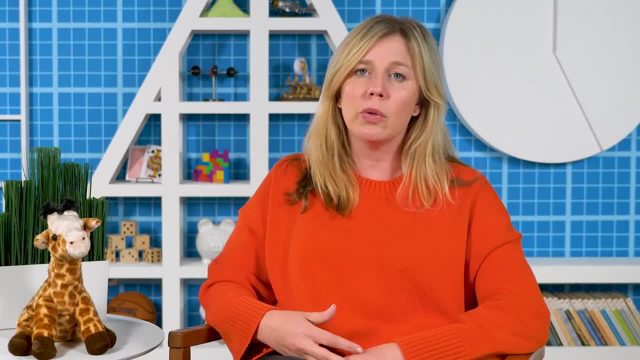 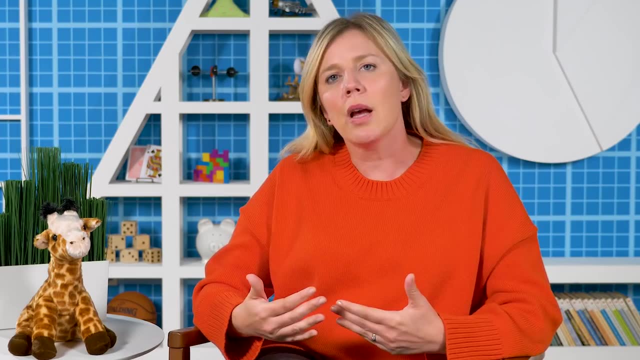 but it's better than a 0.19,, which is in turn better than a 0.20, and on and on. However, in null hypothesis significance testing, p-values need a cutoff. We could set a cutoff at 0.05 and say that a p-value that is less than 0.05 is sufficient. 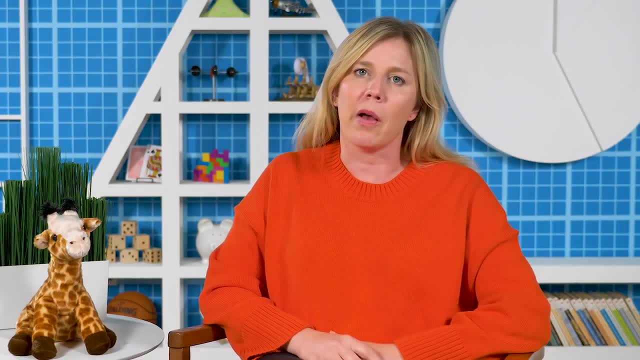 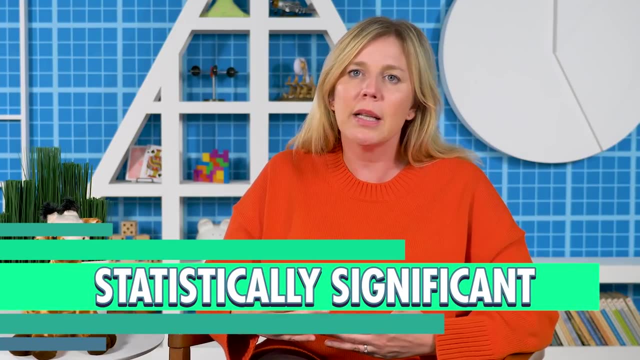 evidence to allow us to reject the idea that the null hypothesis is true. When we can reject the null hypothesis, we consider our results to be statistically significant, which is basically a phrase that just means unlikely due to random chance alone. As we'll see later on, it doesn't. 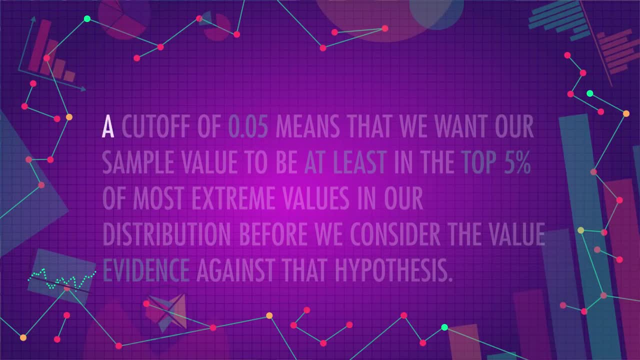 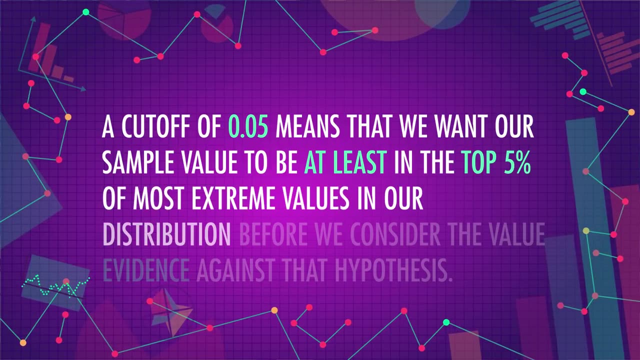 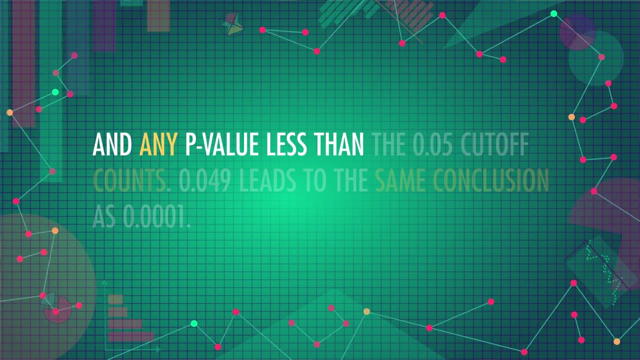 always mean that it should be significant or meaningful to you. A cutoff of 0.05 means that we want our sample value to be at least in the top 5% of most extreme values in our distribution before we consider the value evidence against that hypothesis An any p-value less than the. 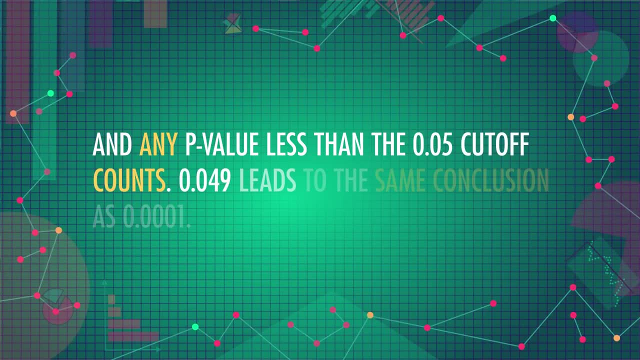 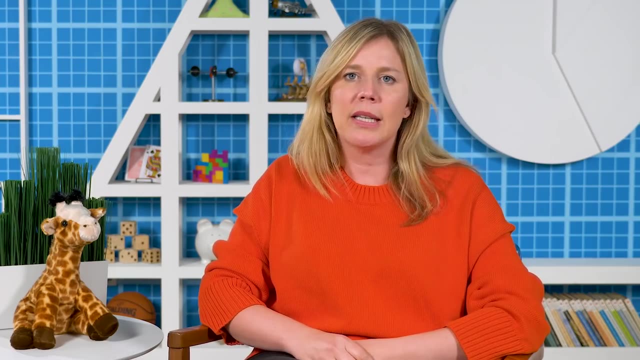 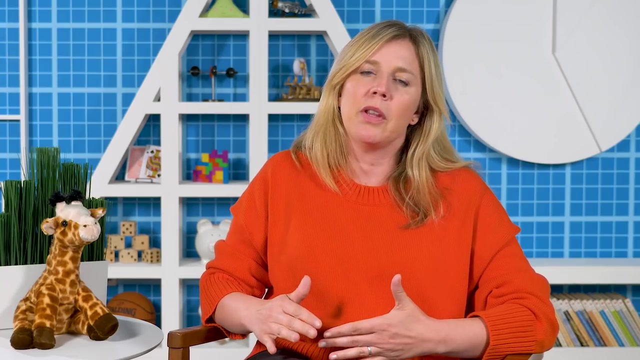 0.05 cutoff counts. 0.049 leads to the same conclusion as 0.0001.. Both cause you to reject the null hypothesis. The current scientific consensus in most fields is that your cutoff, or alpha, should be 0.05.. But there's huge disagreement in the field of.